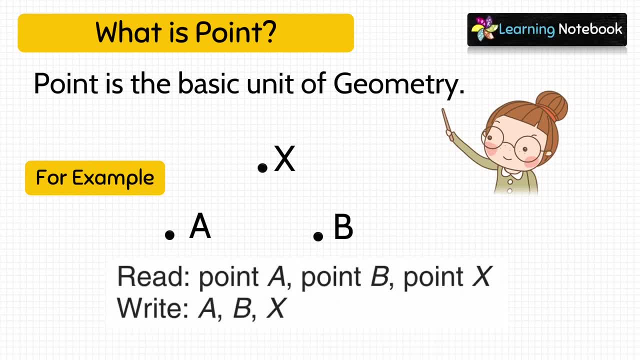 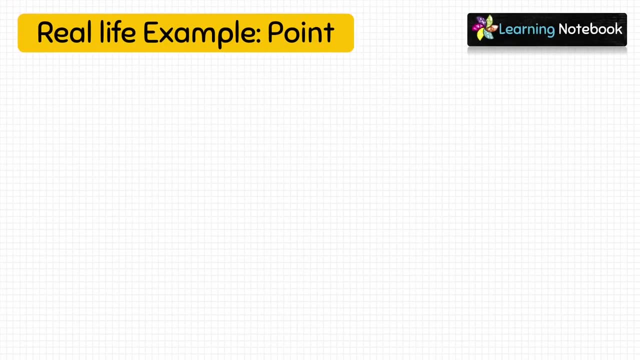 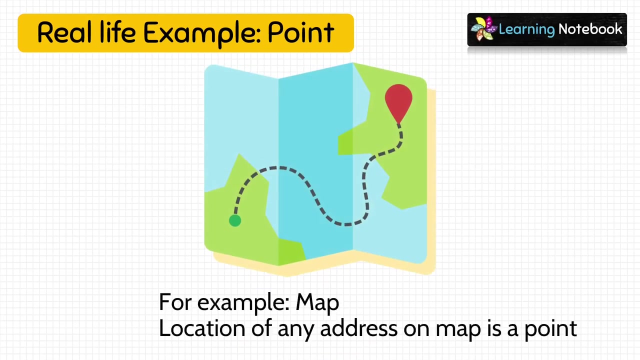 read this As I just told you. we will read them as point A, point B and point X. And how do we write these points? We will write them as A, B and X. Let me tell you a real life example of a point. For example, location of any address on map is a. 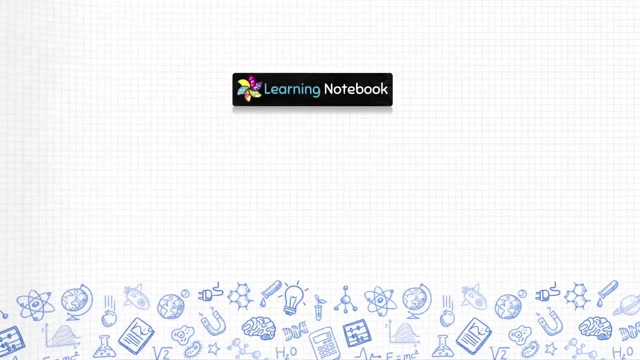 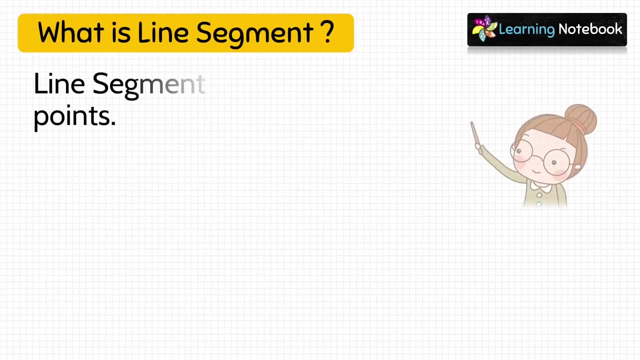 point Next is line segment. A line segment is a straight path between two points. It is the shortest distance between two points. So it is the shortest distance between two points. So it is the shortest distance between two points. For example, there are two points, D, E, So line. 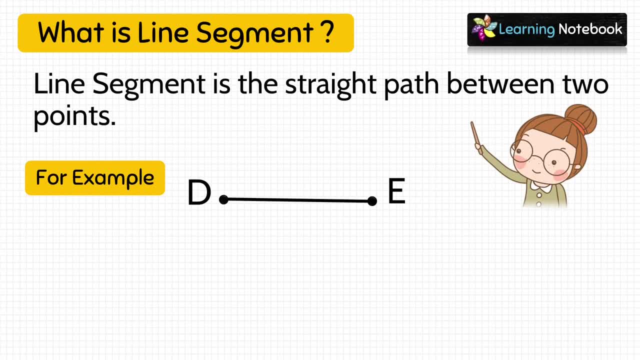 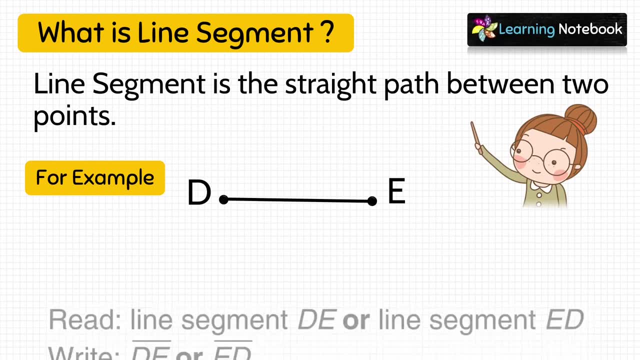 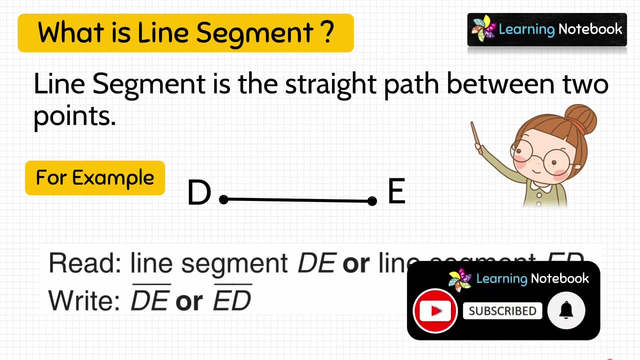 segment is the straight path between these two points. Now let me show you how to read and write line segment. We will read it as line segment D- E or line segment E- D. Both the ways are fine. Similarly, we can either write it as D- E or E- D, with a small line segment on it. Also, students do. 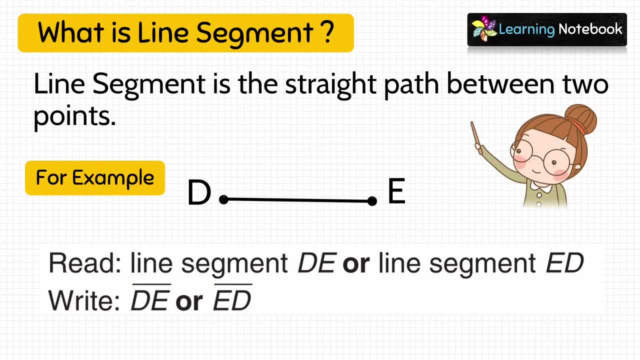 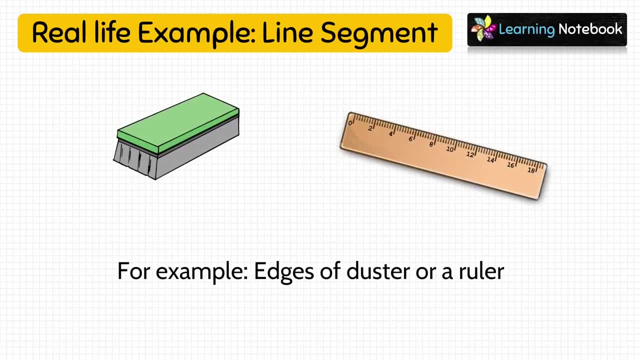 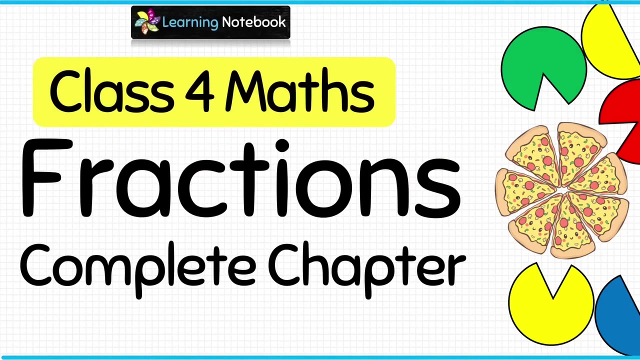 remember that a line segment has a definite length. Now let's see some real life examples of line segment: Edges of duster or edges of a ruler. They are line segment Because of the line segment. they have a definite length. Students, we have a video on complete chapter of fractions. I am 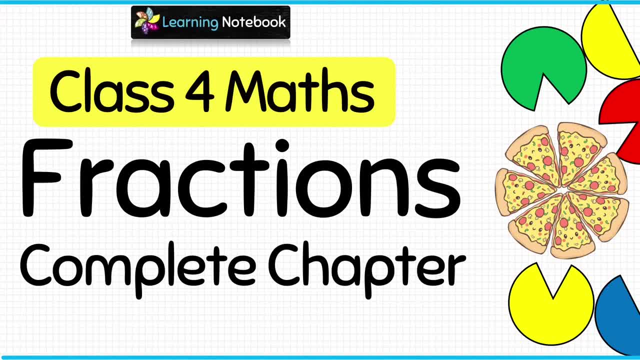 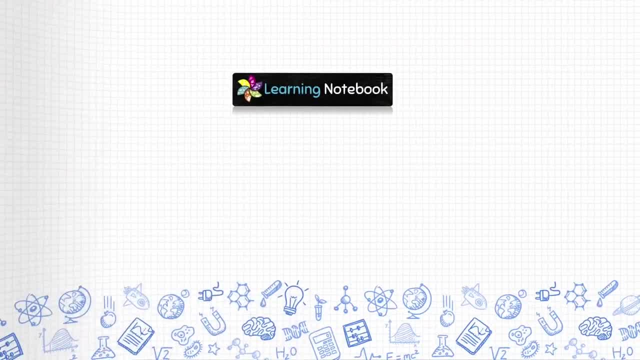 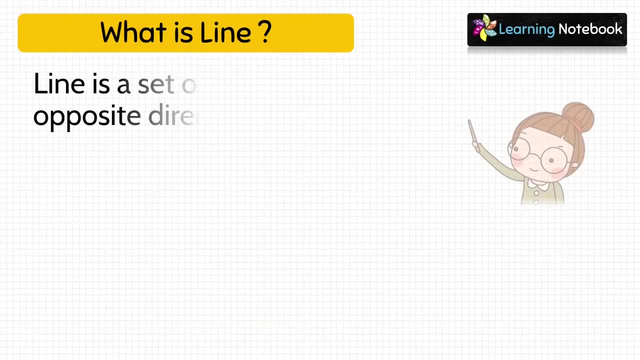 sure all your doubts related to fraction could be resolved after watching this video. The link to this video is below in the description box. Now let's understand what is line. A line is a set of points which extends forever in opposite directions. For example, this is a: 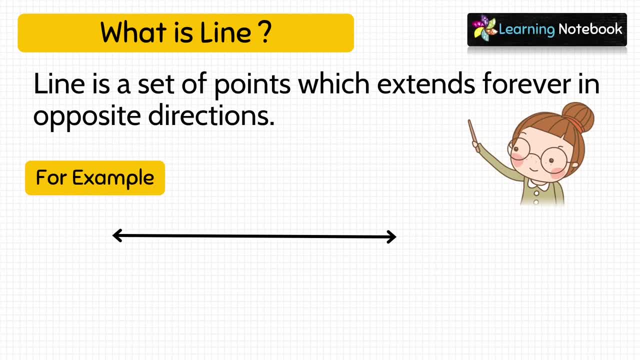 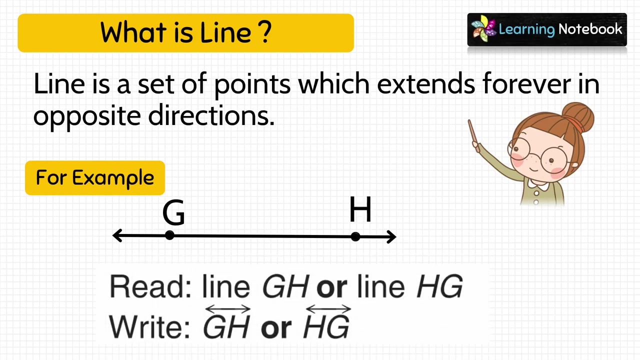 line. The arrow on its both sides represent that a line goes indefinitely in both the directions. So, students, it means a line has no fixed length. Now let me tell you how to read and write a line. For this we need to take two points. Let's take G and H, So we read a line as: 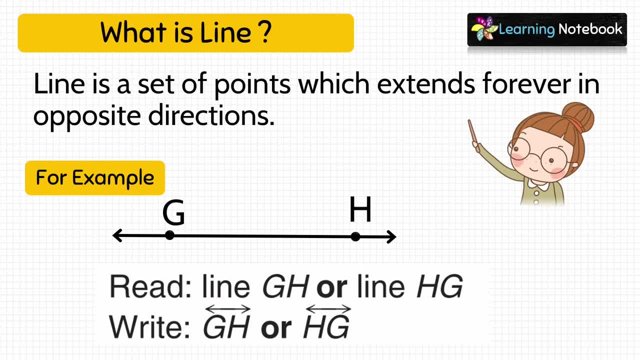 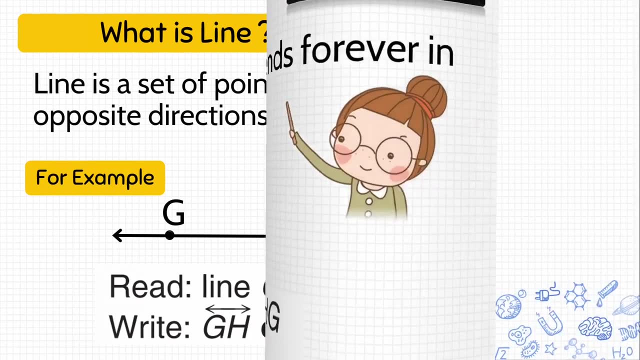 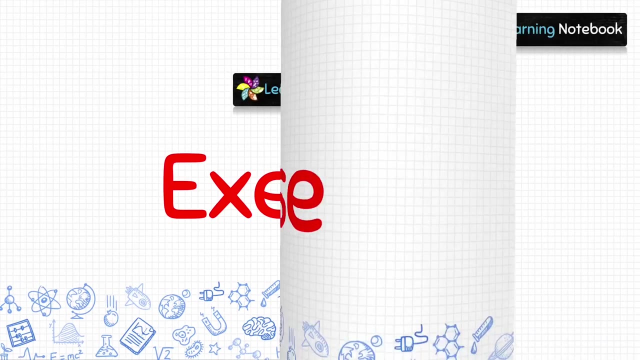 line GH or line HD. Both the ways are fine. Similarly, we can write it as GH or HD, with a small line drawn on it. Now, students, to revise these concepts, let's do an exercise Here. we need to identify line and line. 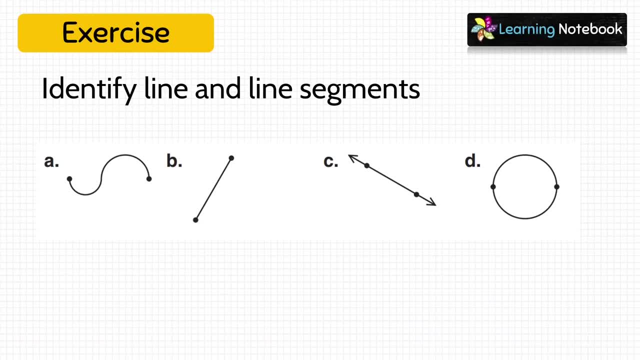 segments. First take a look at figure A. A is not a straight path, So it is neither a line segment nor a line. Now take a look at figure B. It has two endpoints and has a definite length, So it means it is a line. 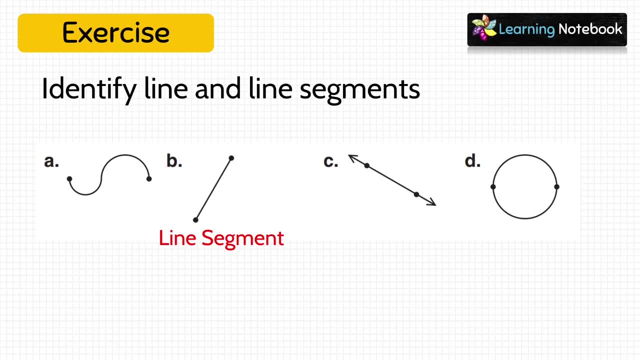 segment. Next, look at the figure C. It has two arrows, So it means it is never ending. Therefore it is a line. And look at the first figure Again. the last figure is not a straight path, So it is neither a line segment nor a line. 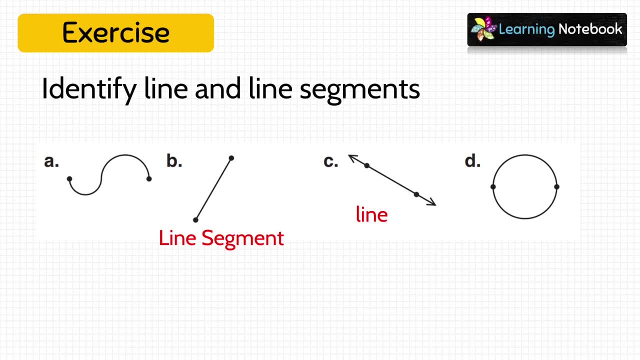 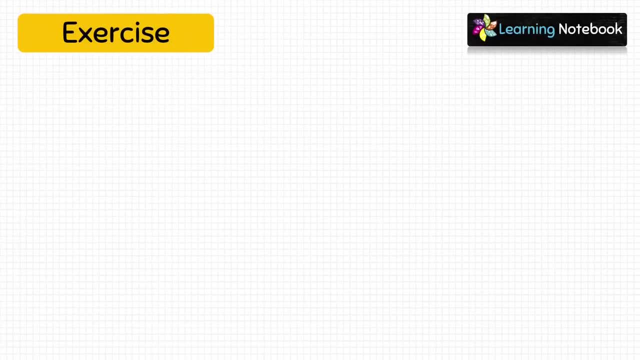 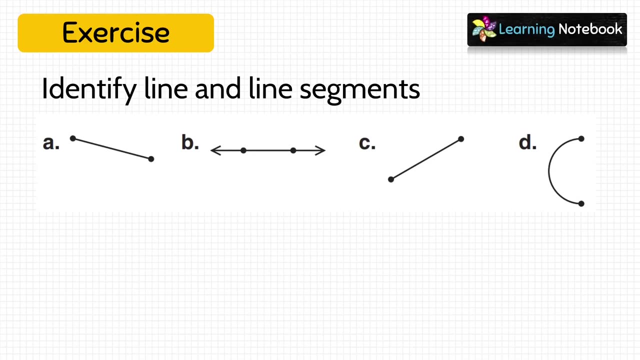 So, students, now I hope you have understood the difference between line and line segments. Now let's do one more exercise. Here again, we need to identify line and line segments. Look at figure A. A is not a straight path, So it is nieather a line segment nor a line. 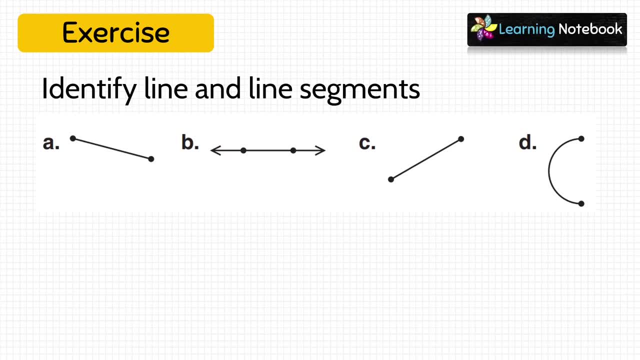 A, can you tell me whether it is a line or a line segment? Yes, it is a line segment because it has two end points. Now, what about figure B? It is a line because it has two arrows, So it means it is never ending. 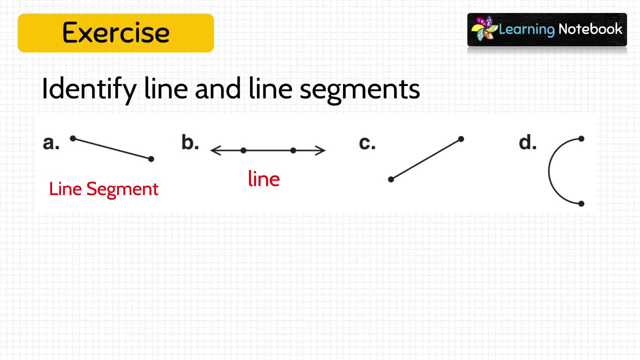 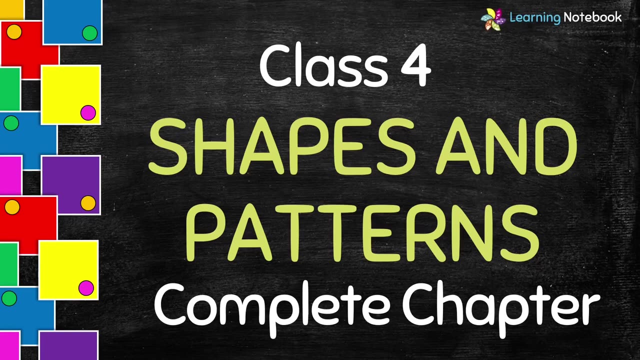 Now let's move to figure C. Again, this is a line segment. Now what about figure D? It is not a straight path, So it is neither a line nor a line segment. Students, we have a separate video on complete chapter of shapes and patterns. 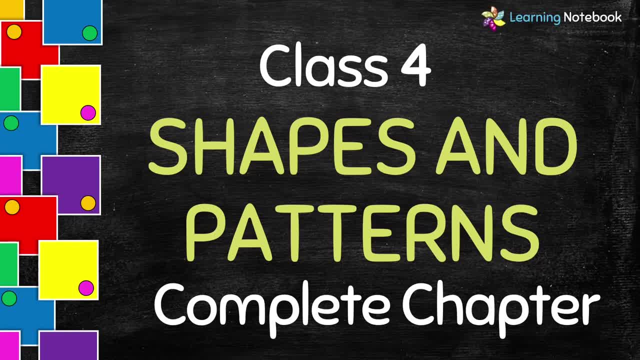 I am sure all your doubts related to this chapter would be resolved after watching this video And also notice that we have lots of quizzes and worksheets available on our channel for each chapter for class 4.. So do check out them on our channel. 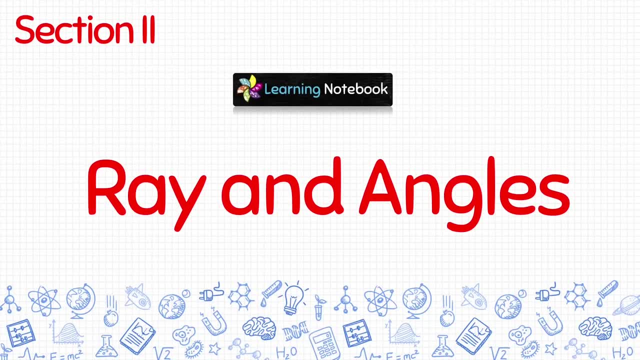 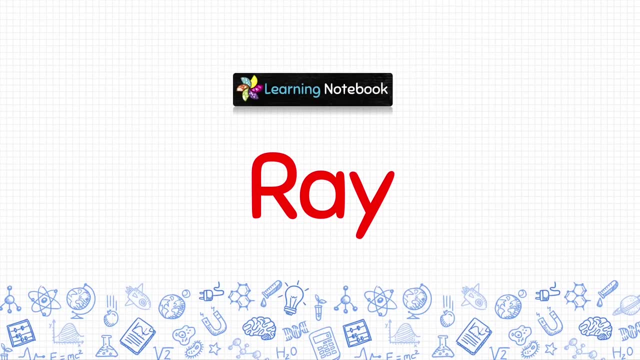 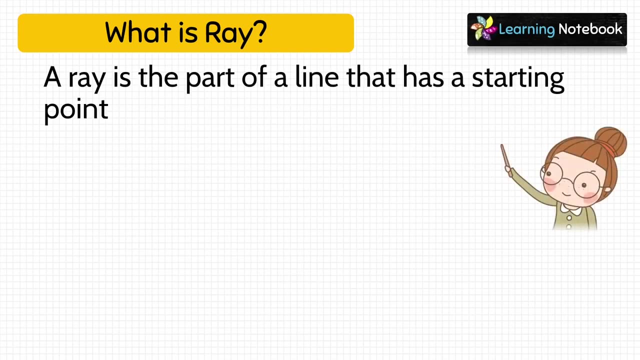 Now let's do section 2, Rays and Angles. First let's understand what is a ray. A ray is a part of the line that is a line segment. It is a line segment that has a starting point and it goes on forever in one direction. 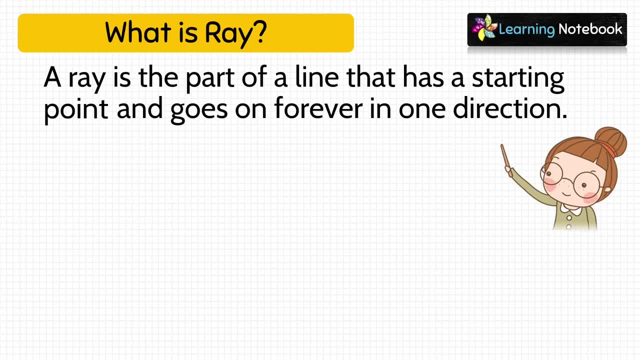 It means ray also has no fixed length. It cannot be measured. For example, this is a ray. It has a starting point called K and it goes indefinitely in one direction, towards J. Now let me show you how to read and write ray. 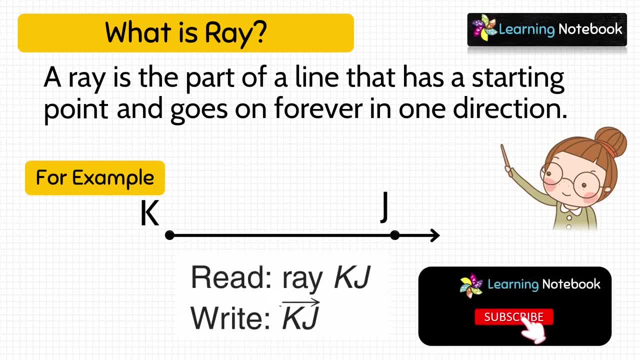 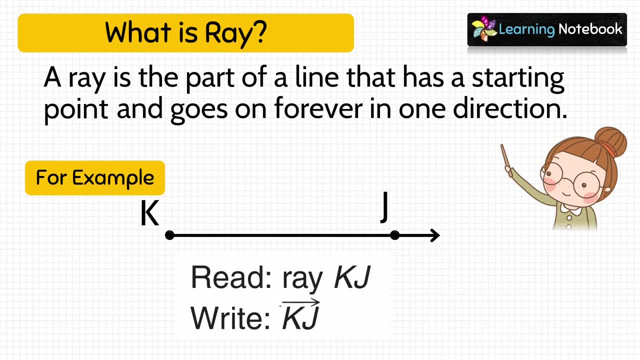 We will read the starting point first, So it will be read as ray KJ. Thus, students, there is only one way to read ray. That is by reading the starting point first. And now how to write it. We will write it: KJ. 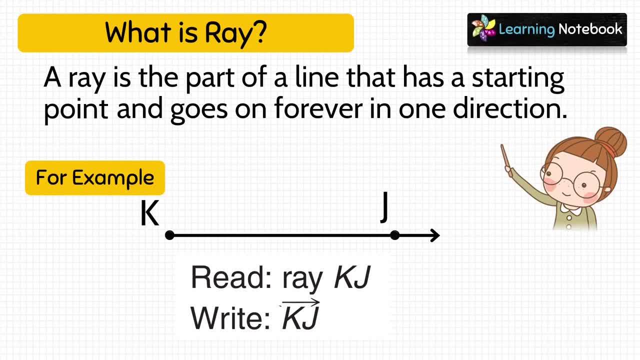 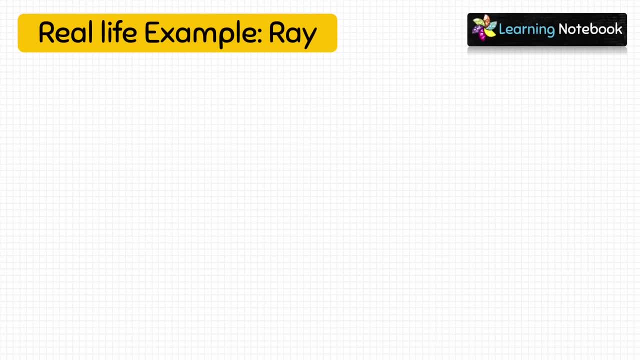 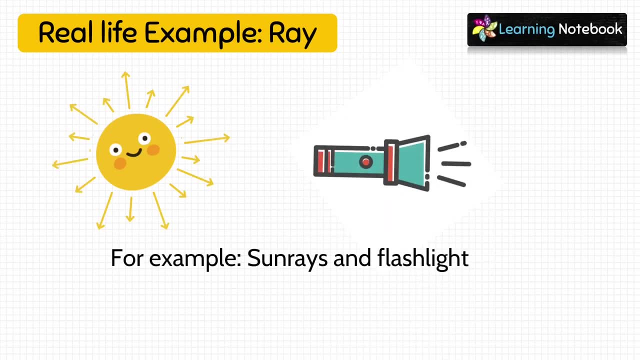 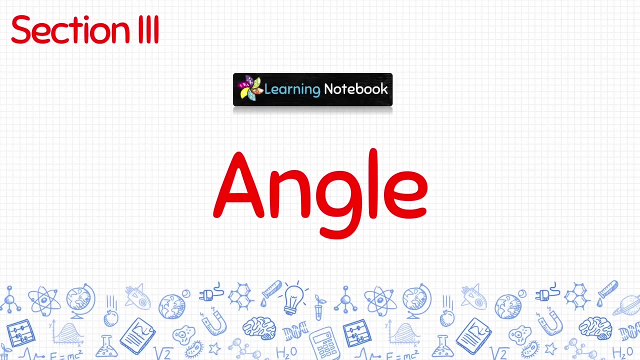 With a small ray drawn over it. Now let's see some real life examples of ray: Rays from sun and rays from flashlight. These are examples of ray Because they have a starting point and they go indefinitely in one direction. Now, in section 3, we will learn about angles. 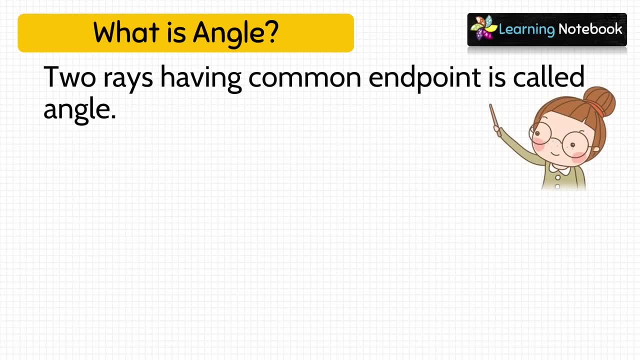 Two rays having a common end point is called angle. For example, here ray AB and ray AC are forming an angle. The two rays are called arms, honesty, arms of the angle, And the common end point is called vertex of the angle. So, students, 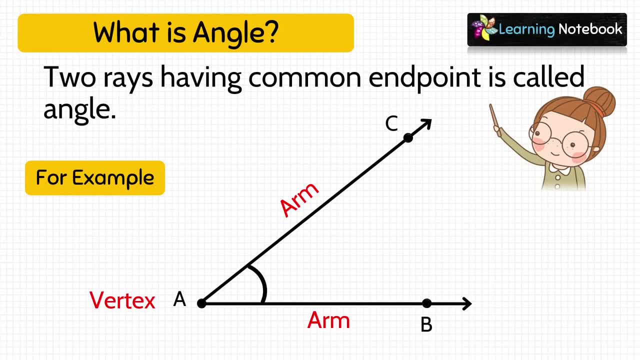 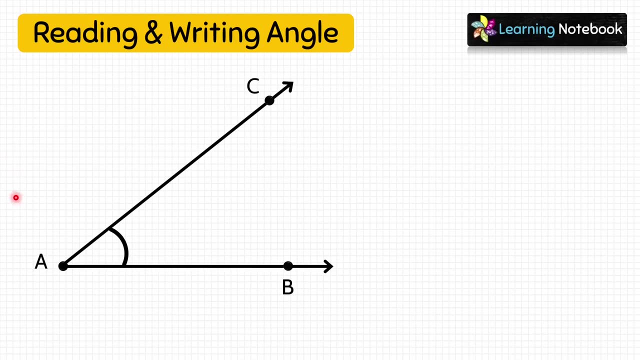 A is the vertex here, while AC and AB are arms of the angle. Now let's learn how to name an angle. To name an angle, we need three points, and the point at which an angle is formed will always be in the middle. Here, angle is formed at vertex A, So A will always. 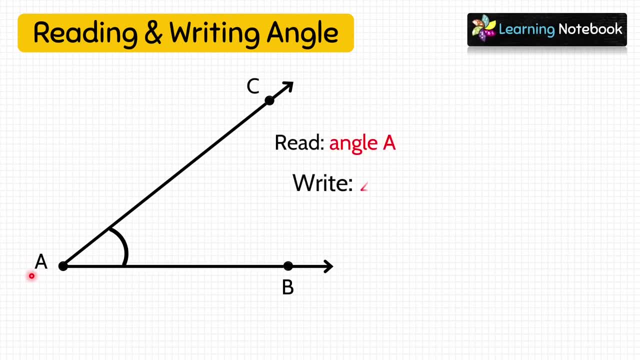 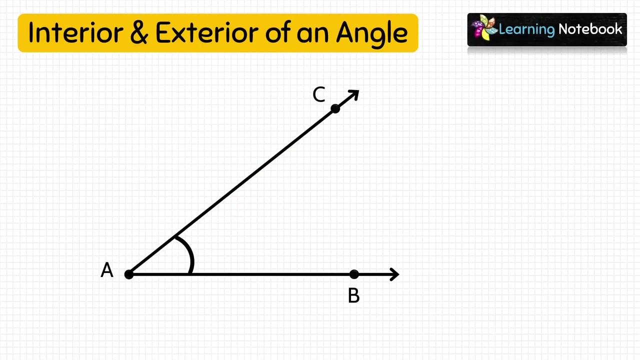 be in the middle while naming this angle, So we can read and write this angle as angle A Or angle CAB or angle BAC. Now let's see what is interior and exterior of an angle. Let's consider an angle CAB, So this shaded region is the interior of angle CAB, while 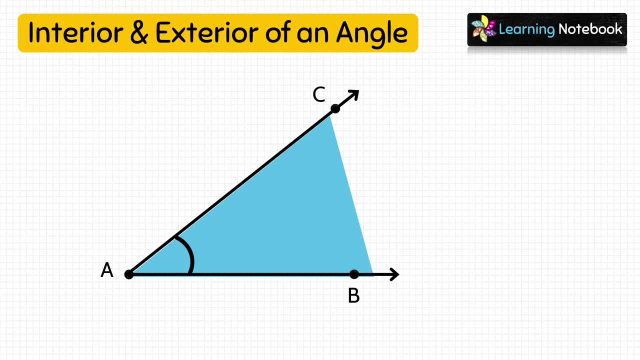 the rest of the interior is the exterior. So the shaded region is the interior of angle area is considered to be exterior of an angle. So let's take a point I. This point lies in the interior of an angle, while the point E lies in the exterior of the angle and other 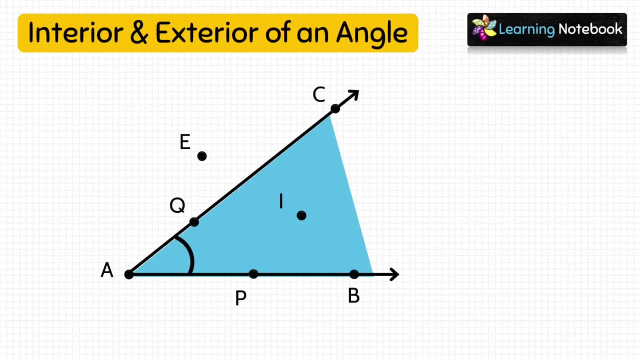 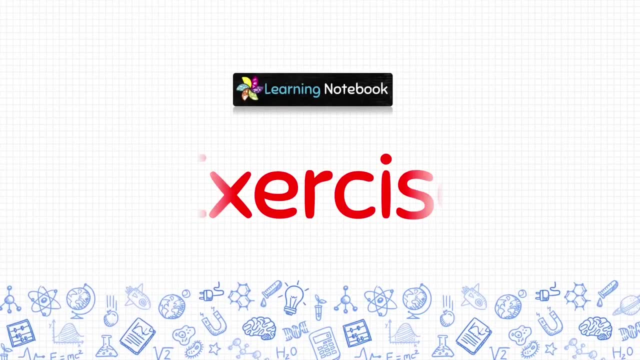 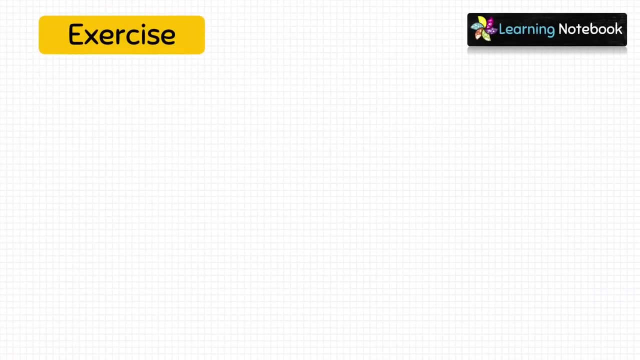 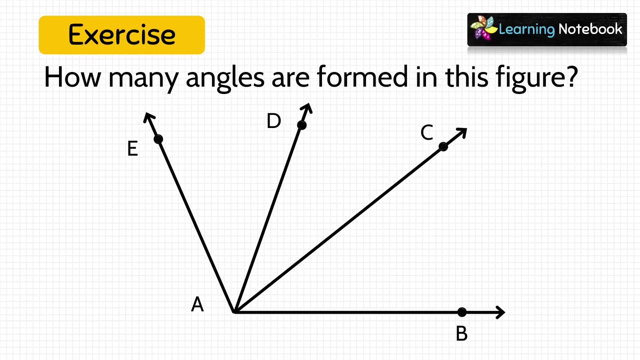 points like P and Q. they lie on the angle CAB. Now to revise these concepts, let's do an exercise. How many angles are formed in this figure, Students? look at this figure carefully. We can see only one angle. How many angles are formed in this figure, Students? 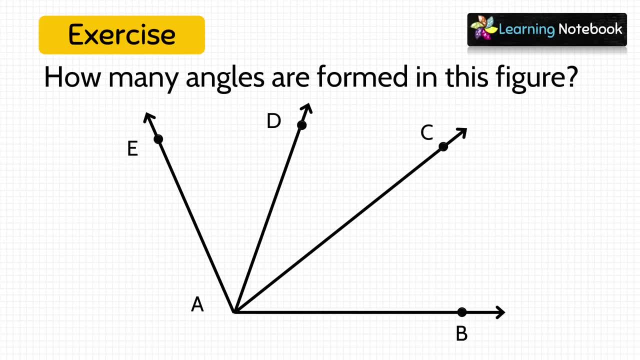 look at this figure. How many angles are formed in this figure. TAES is formed. Threediagonal angle formed in this figure. How many angles are formed in this figure? Robert's Many angles are formed. No, Do we have only 3 angles in this figure or do we have more angles? 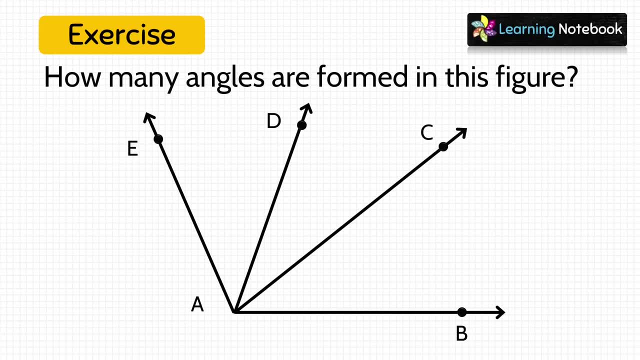 formed in this figure. Let's check it out. First angle which we can see is angle BAC. second angle being formed here is angle CAD and third angle is angle DAS. Now look carefully please. So we will divide power by E, right from 0 to E equal to 0.. This will mos that. 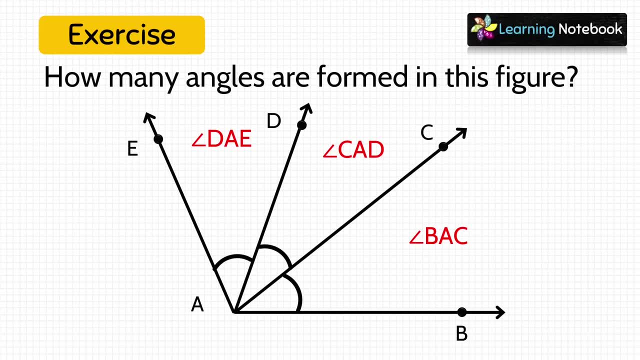 very small angle we have formed here And that part we have shortcut ticking that area along this square sequence right from 0 to 1.. So we will spec frames and see if we can. We have another angle which is called angle CAE. 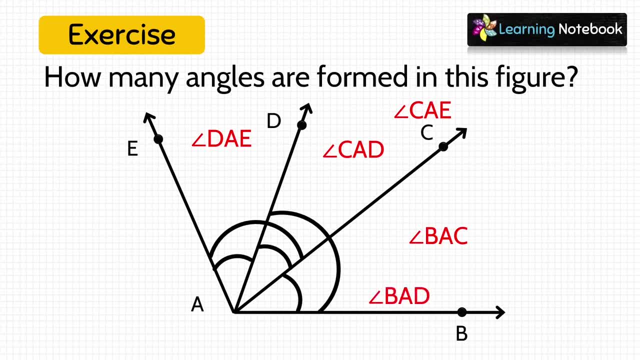 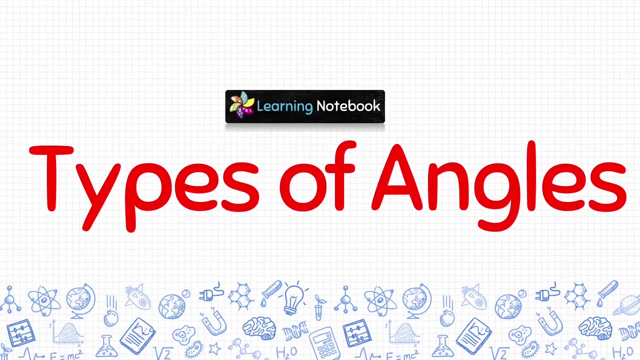 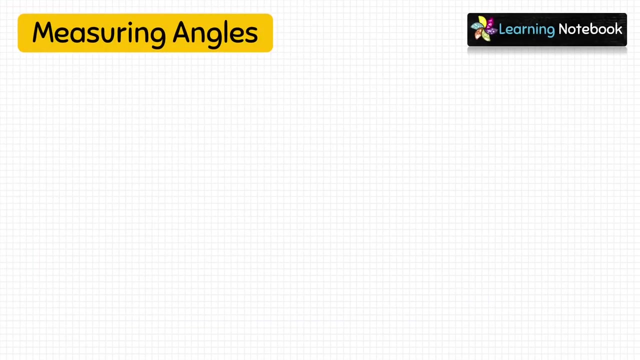 Then fifth angle being formed here is angle BAD, And last angle being formed here is angle BAE. So it means six angles are being formed in this figure. Now let's learn about types of angles. First, let me tell you a little bit about measuring angles. 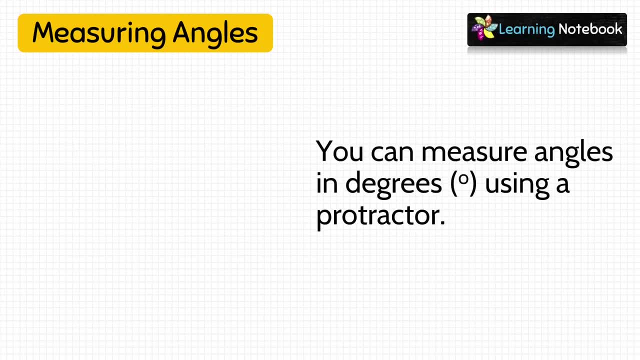 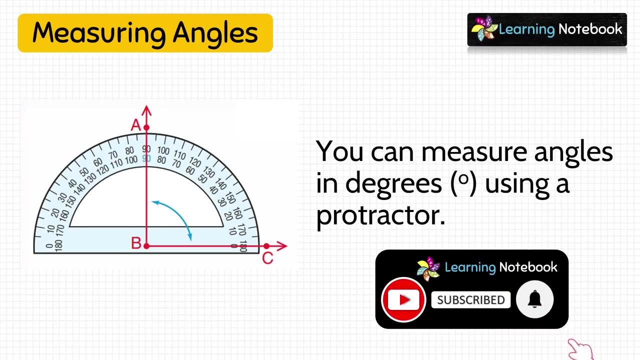 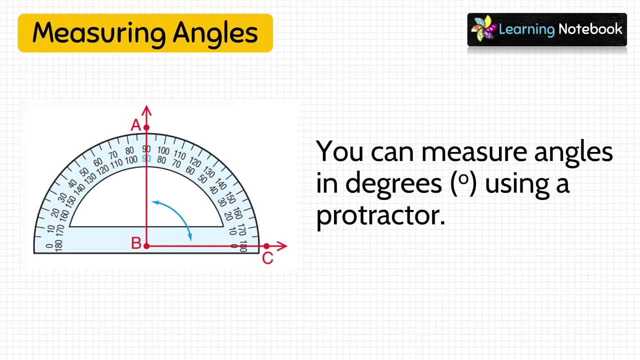 Measure of an angle is the distance between its two arms. You can measure angles in degrees Using a protector. We will learn how to measure angles using a protector in another video, But for now you understand that angle is measured in degrees. Now let's learn types of angles. 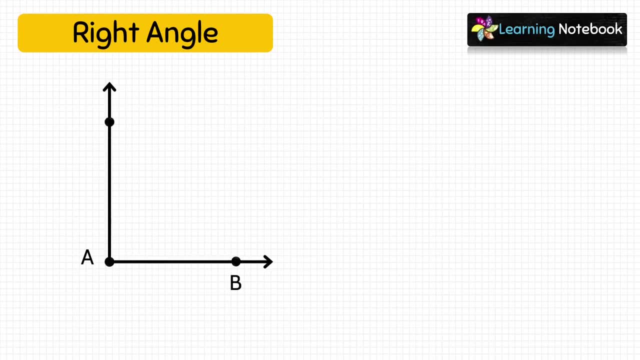 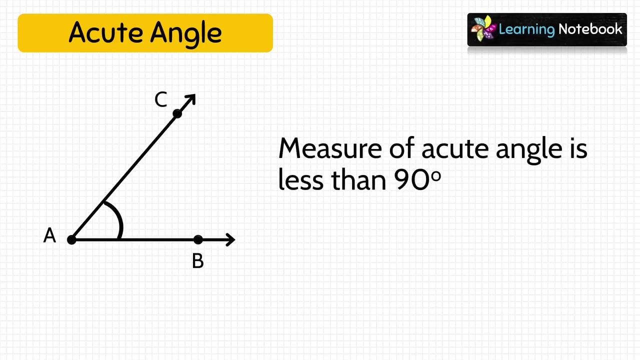 First is right angle. The measure of right angle is 90 degree, as shown here. This is a right angle. Now, next type of angle is acute angle. As you can see, this angle measures less than 90 degree. So measure of acute angle is always less than 90 degree. 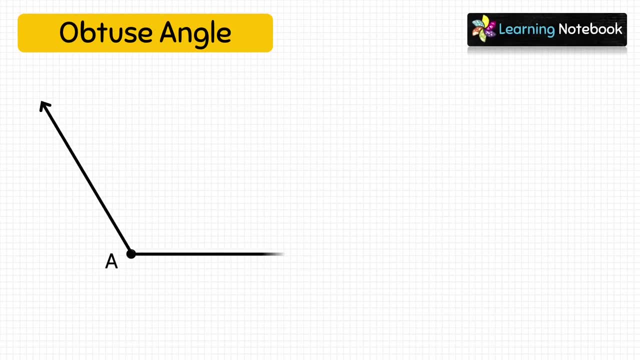 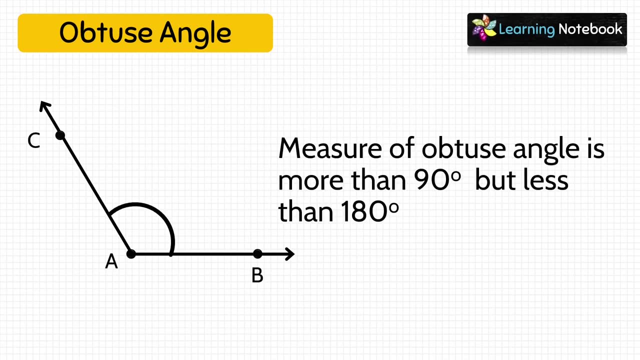 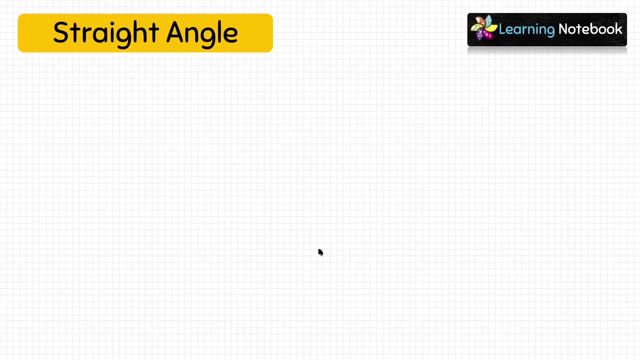 The third type of angle is opposite angle. The third type of angle is opposite angle. Measure of obtuse angle. Measure of obtuse angle is more than 90 degree but less than 180 degree. And the last type of angle is straight angle. 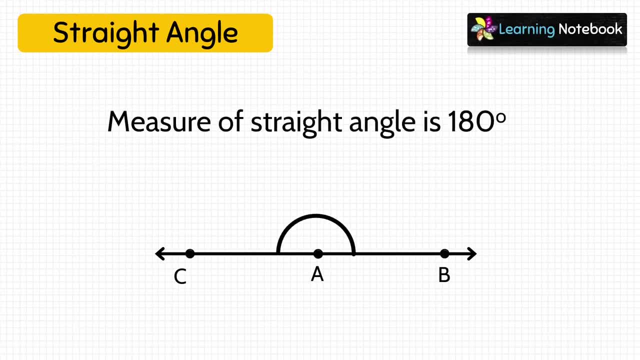 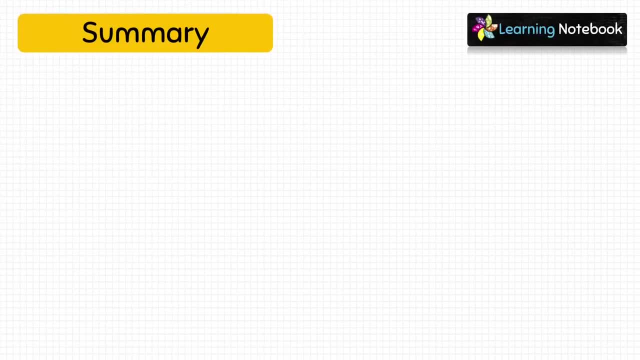 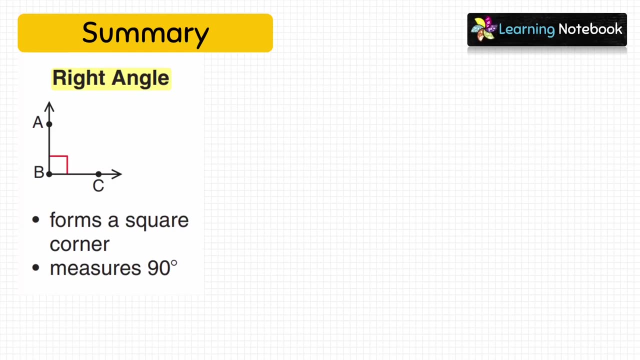 The measure of straight angle is exactly 180 degree, as you can see here, And the last type of angle is straight angle. Now let's summarize types of angles. First is right angle, which measures exactly 90 degree, and it forms a square corner. 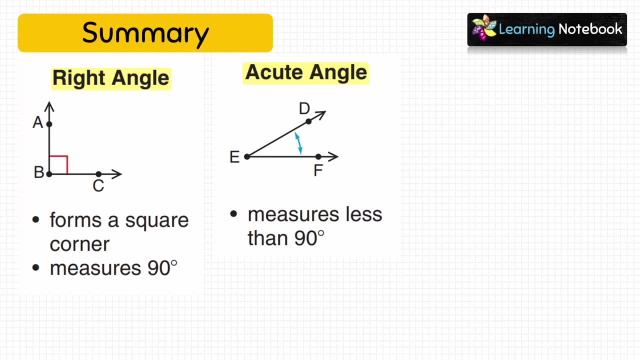 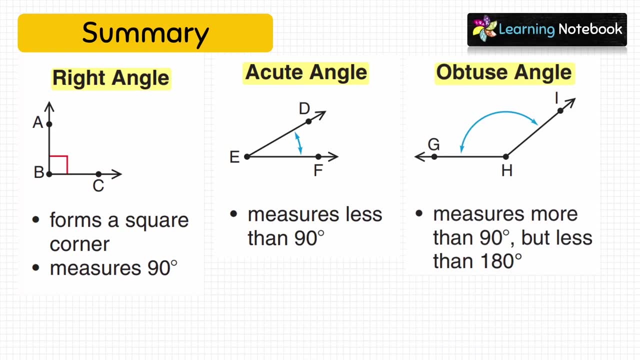 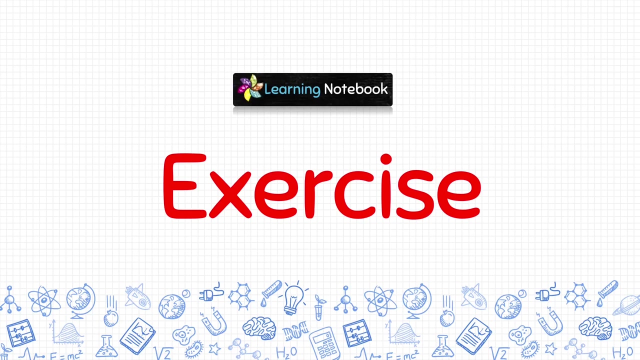 Second is acute angle, which always measures less than 90 degree. Third type is obtuse angle, which measures more than 90 degree but less than 180 degree. And the last type of angle is straight angle, which measures exactly 180 degree. Now, students, let's do an exercise based on types of angles. 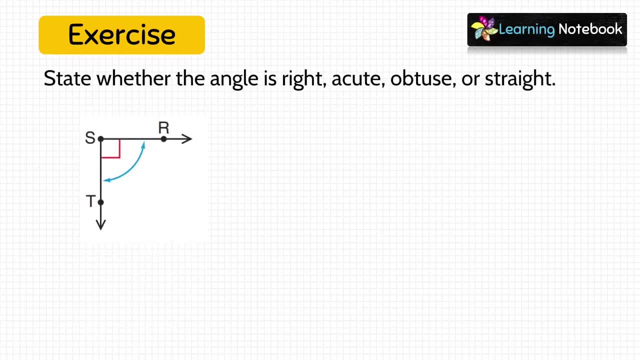 Question is: state whether the angle given below is right, acute, obtuse or straight angle. Students, as you can see, the angle given below is right. As you can see, this angle measures exactly 90 degree, So it is a right angle. 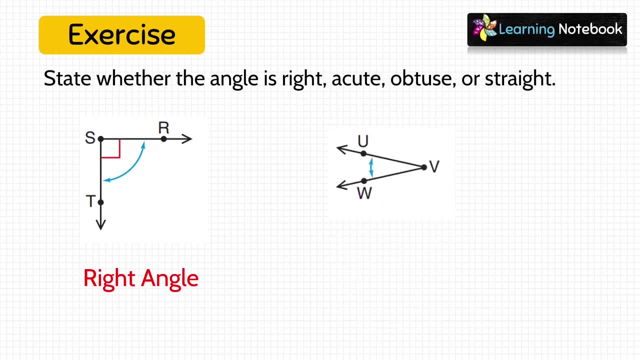 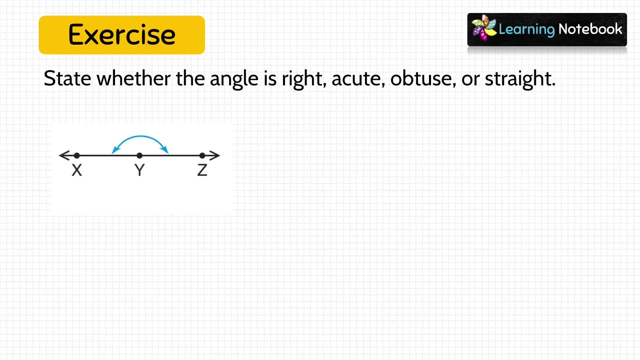 Let's see the next figure. Here the angle measures less than 90 degree, So it will be an acute angle. Now have a look at this figure. Here the angle measures exactly 180.. So it is a straight angle. 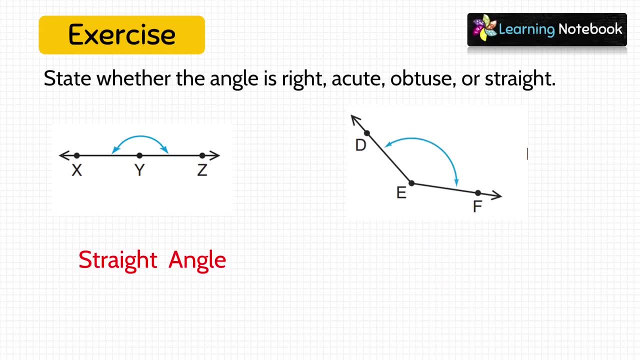 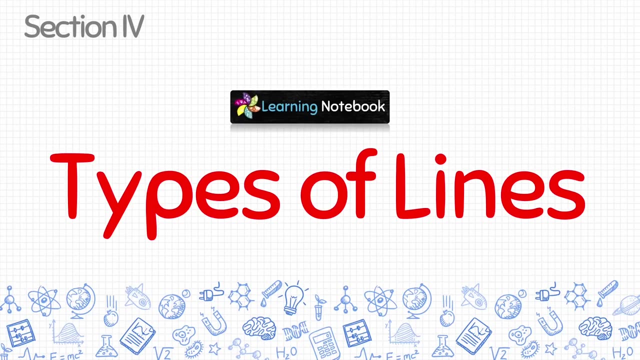 Now let's see the next figure. Here, the angle measures more than 90 degree, but less than 180 degree, So it is an obtuse angle. Now let's understand types of lines. Let's understand types of lines. 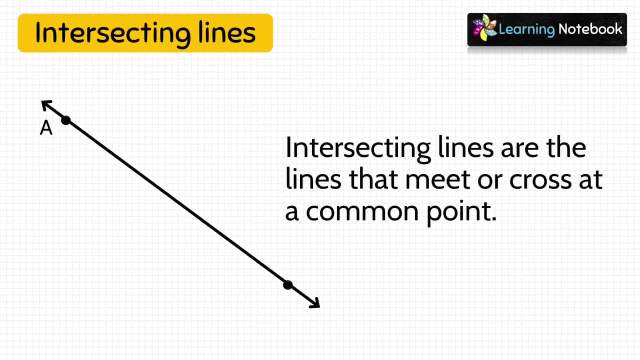 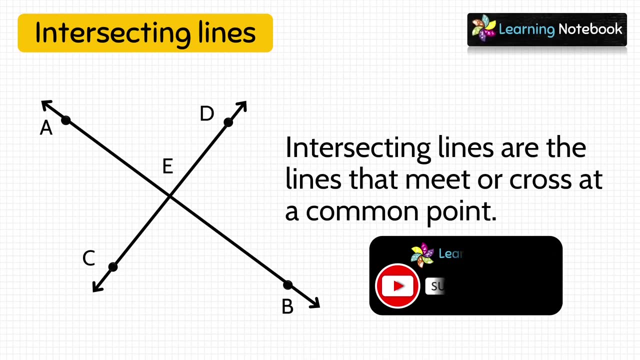 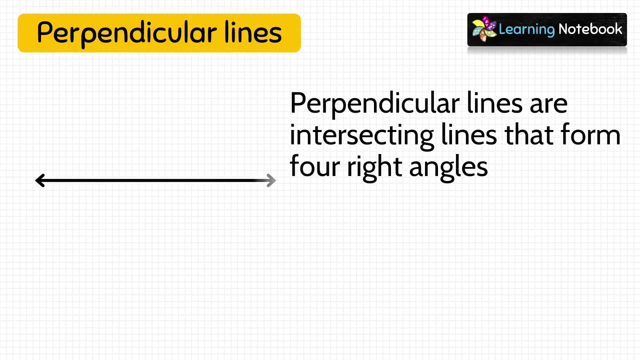 First type is obtuse angle Intersecting lines. Intersecting lines are the lines that meet or cross at a common point, Like here: line AB and line CD are intersecting at a common point. E. Next type is perpendicular lines. Perpendicular lines are also intersecting lines, but they 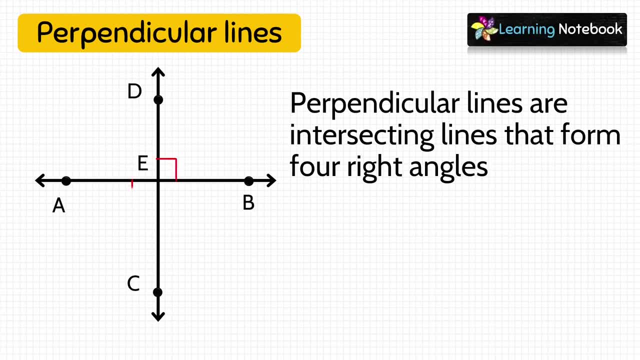 intersect to form foreright angles. As you can see here, line CD is perpendicular to line AB and they are intersecting at point E to form foreright angles. We have a special symbol to denote perpendicular lines, so we will write: line CD is perpendicular to line AB. 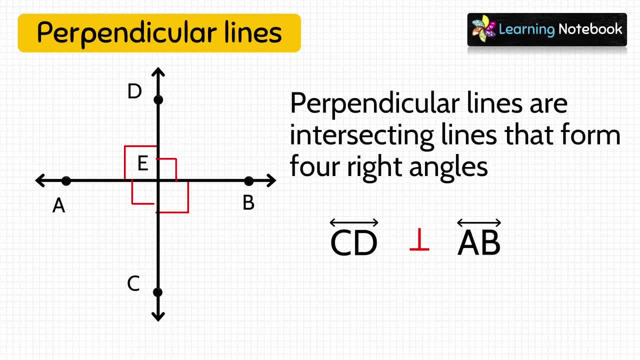 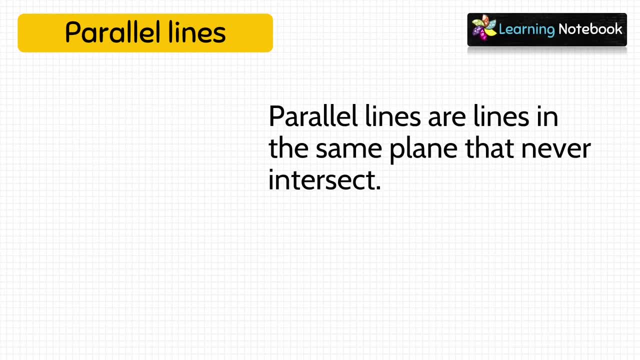 So this is the symbol of perpendicular lines. Now, third type of lines are parallel lines. Parallel lines are lines in the same plane that never intersect. As you can see on the screen, line AB and line CD are parallel lines. They will never intersect each other. 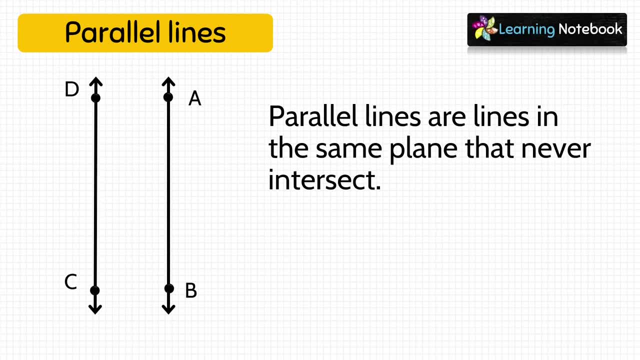 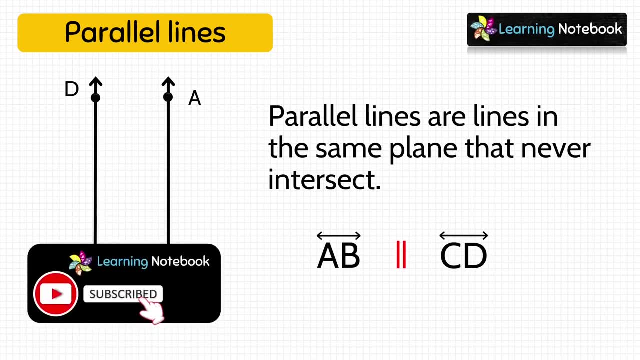 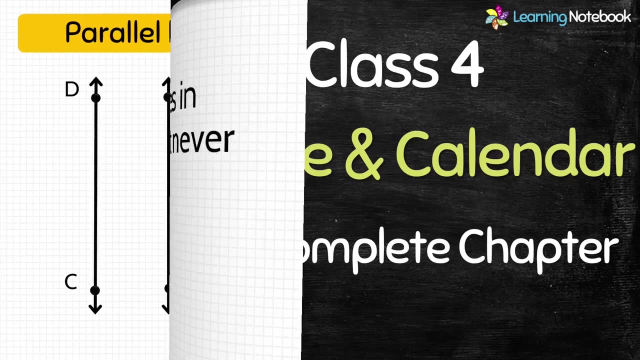 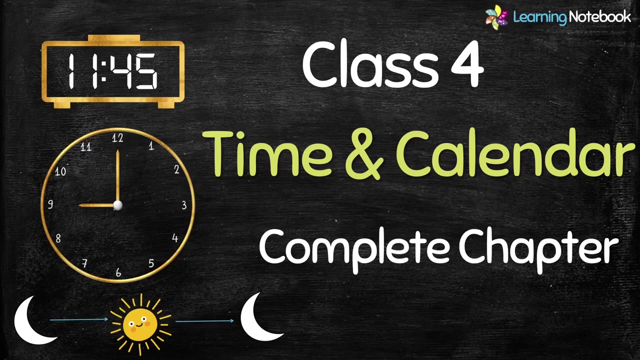 Remember we have a special symbol to denote parallel lines. So we will write: line AB is parallel to line CD, So this symbol in red is a symbol of parallel lines. Students, we have a separate video on complete chapter of time and calendar for class 4.. 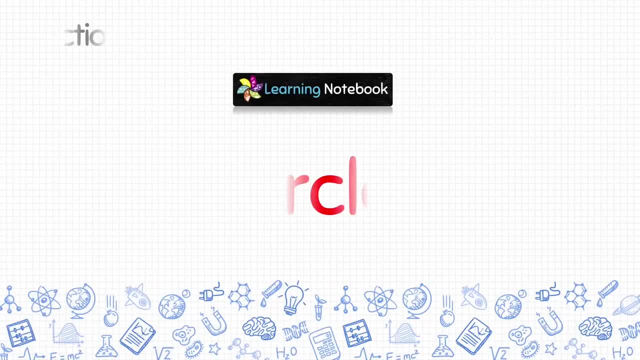 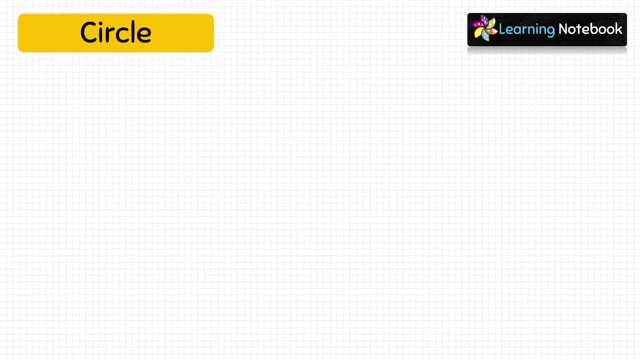 Do watch this video Now. our next topic is circles. Students, this is a circle. Some of the real life examples of a circle are button, pizza, donuts, etc. The middle point of a circle is called center, As you can see in this figure. 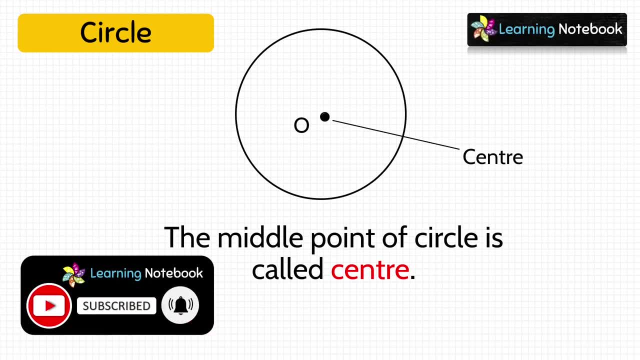 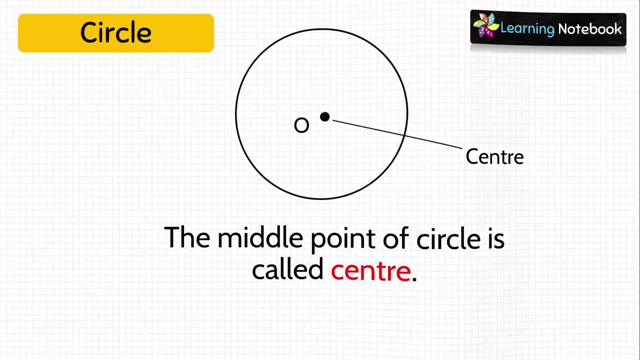 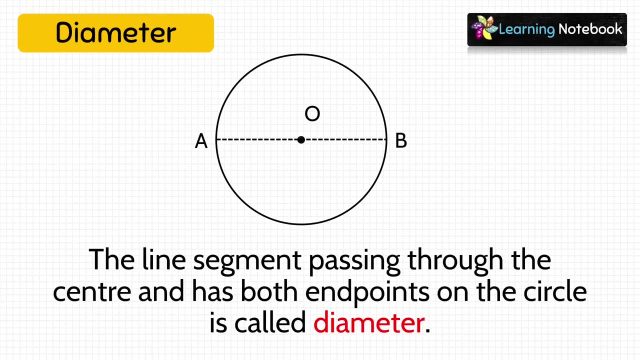 This is a center of the circle, And center of the circle is usually denoted by capital letter O. Now let's understand what is diameter. The line segment passing through the center and has both endpoints on the circle is called diameter of the circle. 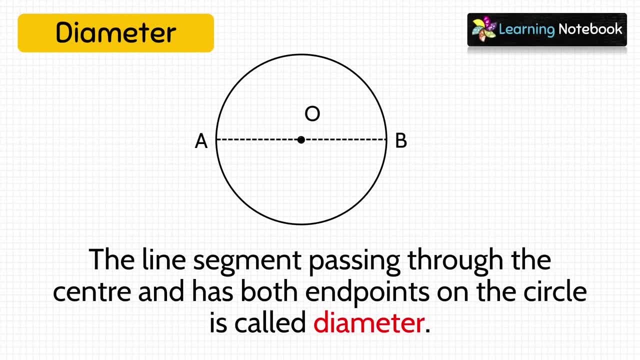 Like here, AB is the diameter, So the diameter of this circle, as it is passing through the center and has both endpoints, A and B, on the circle, Students do remember the diameter of a circle can be drawn horizontally, vertically or even slanting lines. 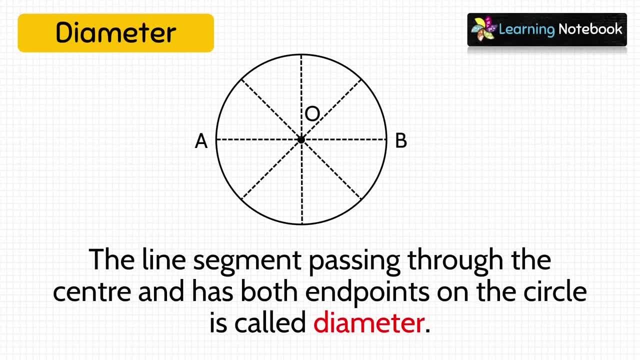 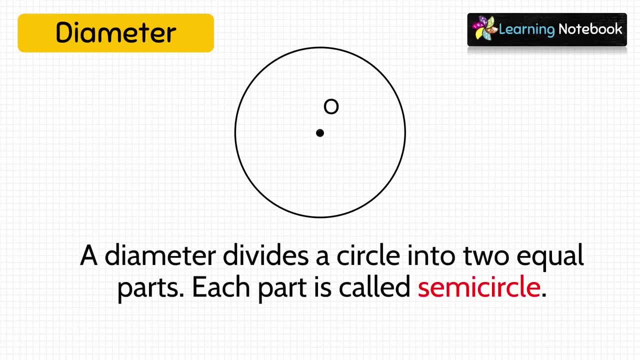 But it should always pass through center of the circle. A diameter divides a circle into two equal parts, And each part is called semi-circle. Like here, this diameter is dividing the circle into two semi-circles. Similarly, this vertical diameter divides the circle into two semi-circles. 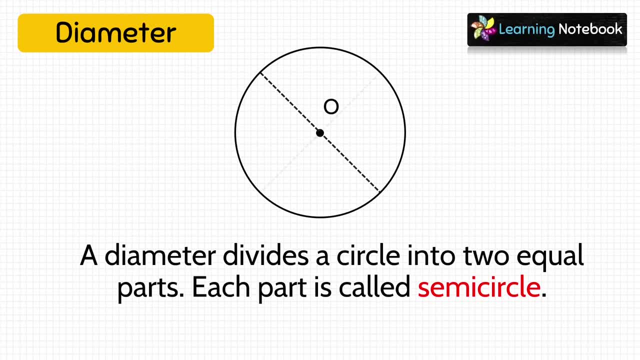 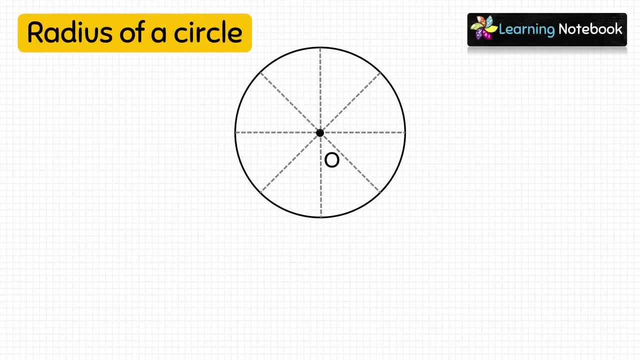 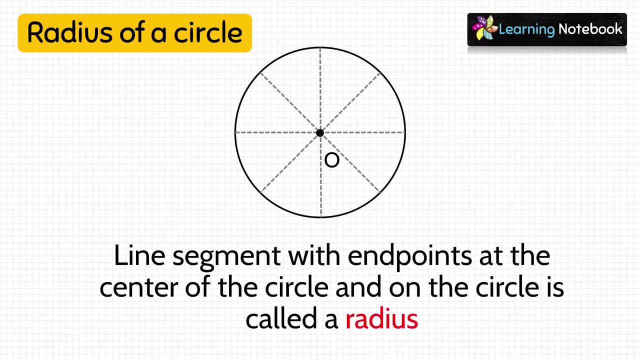 And in the same way the slanting diameters divide the circle into two semi-circles. two semicircles Now. what is radius of a circle? A line segment with endpoints at the center of the circle and on the circle is called a radius. For example, here OA is the radius of the circle. 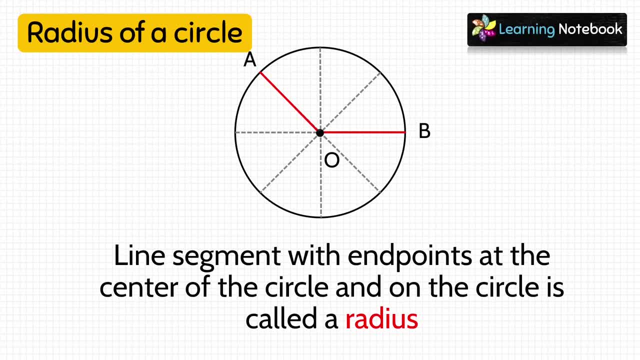 Similarly, OB is also the radius of this circle, because one point is at the center of the circle and other point is on the circle. So, students, it means a circle can have more than one radius. Here, OA, OB, OC, OD, all these are radii of this circle. 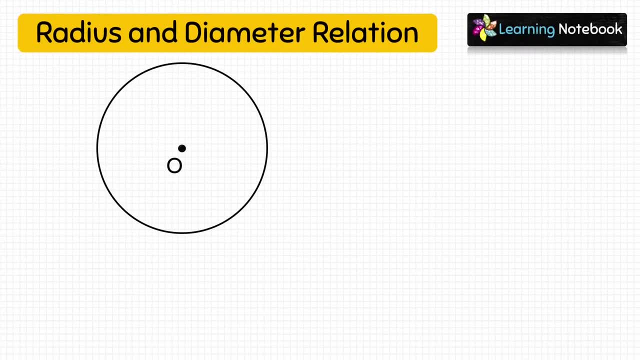 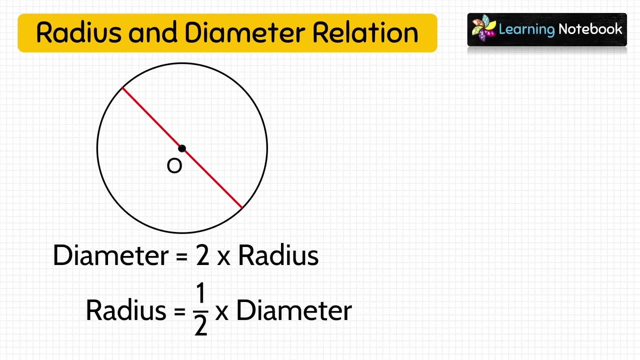 Now let's understand relation between radius and diameter. Diameter equals to 2 into radius. or we can say radius equals to half of diameter. You can easily learn the relationship between diameter and radius with the help of table of two. If radius is 2,, then diameter will be. 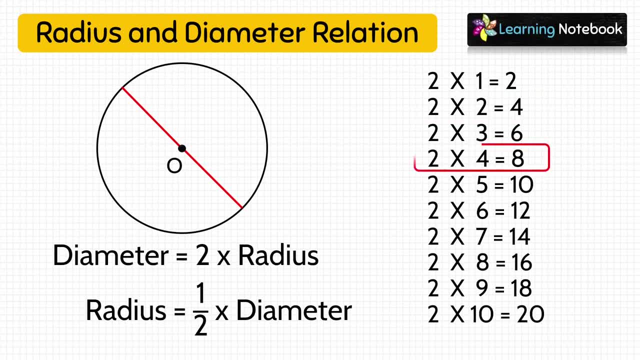 2.. If radius is 2,, then diameter will be 2.. If radius is 2,, then diameter will be 2.. Similarly, if the radius is 4,, then diameter would be twice of 4,, that is 8.. And if radius is 8,. 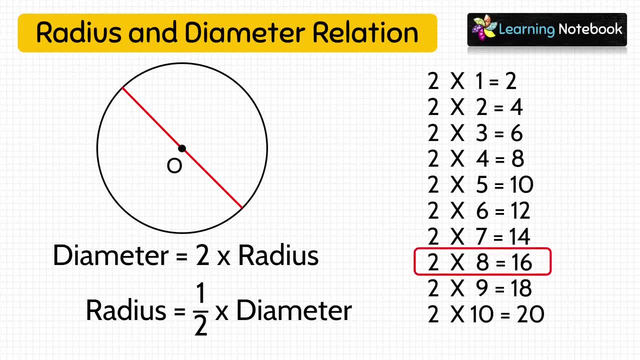 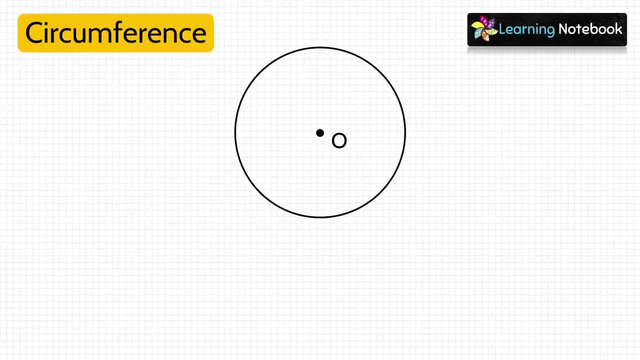 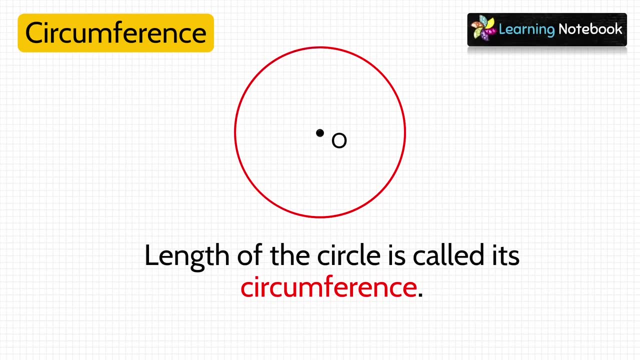 then diameter would be equal to 16.. Now next is circumference. Length of the circle is called circumference. Length of the circle is called circumference. Length of the circle is called circumference. That means the boundary of the circle is called its circumference. 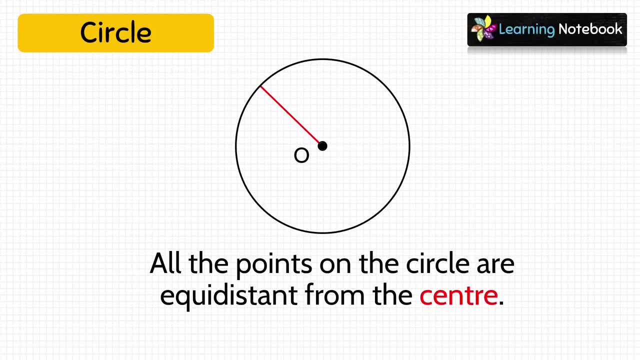 Now students do remember that all the points on the circle are equidistant from the center. Equidistant means at equal distance. So here, all the points on the circle like A, B and C, they are at equal distance. So here, all the points on the circle like A, B and C, they are at equal distance. 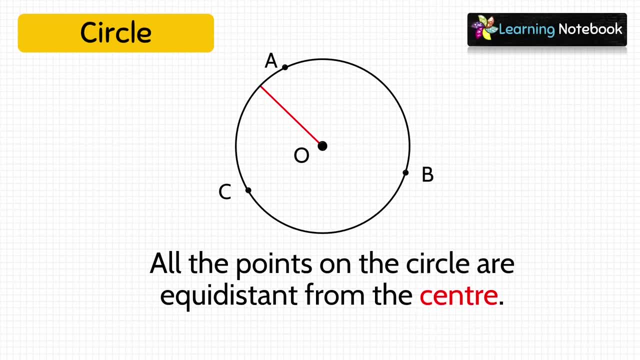 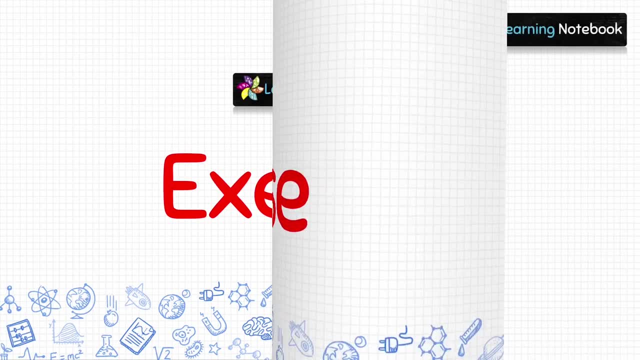 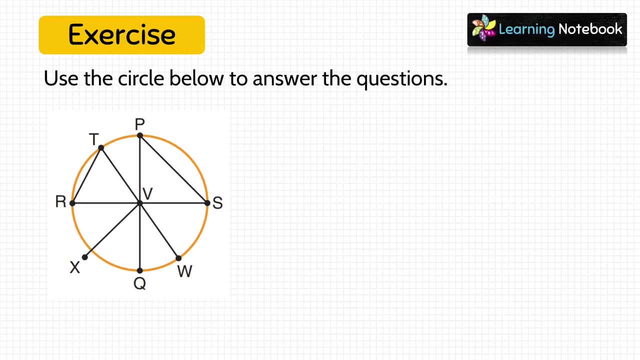 equal distance from center O. Now let's do an exercise based on the concepts of circle. Use the circle below to answer the questions. First question is: name the circle and its center. Remember that a circle is always named by its center. So first let's see. 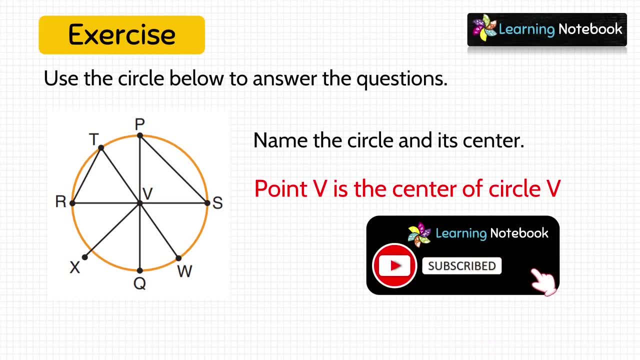 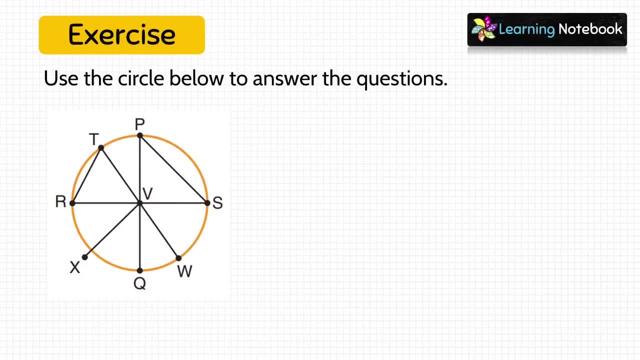 Its center is V, So we will write: point V is the center of circle V. Second question is how many diameters are shown in this circle and name the diameters. So, students, as I told you diameters, they pass through center of the circle and has. 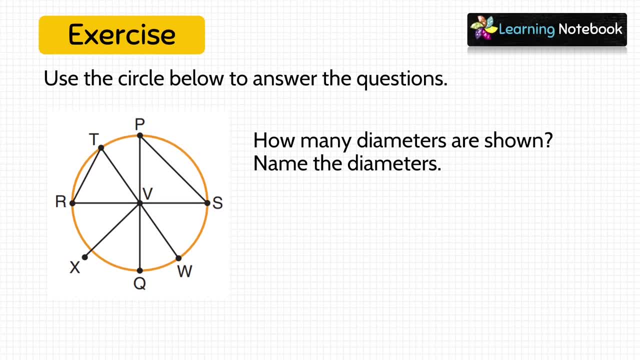 both endpoints on the circle. So let's look for such line segments. We have RS, line segment TW and line segment PQ, So there are three diameters of this circle. Third question is: is TR a radius? Yes, Explain. 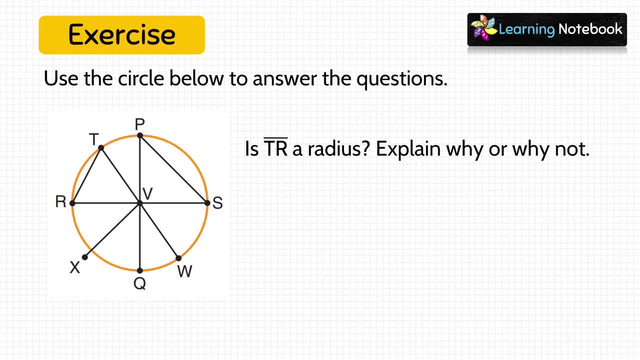 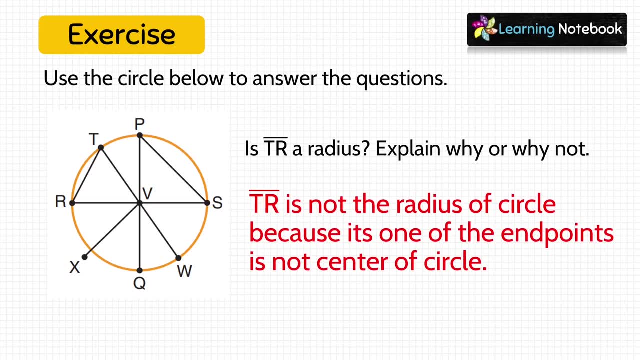 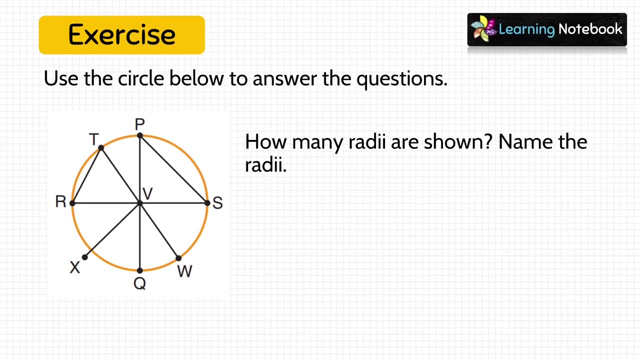 Explain why, or why not, TR is not the radius of a circle, because it's one of the endpoints, is not the center of the circle. And the last question is how many radii are shown here and name the radii. So, first of all, what is radii? 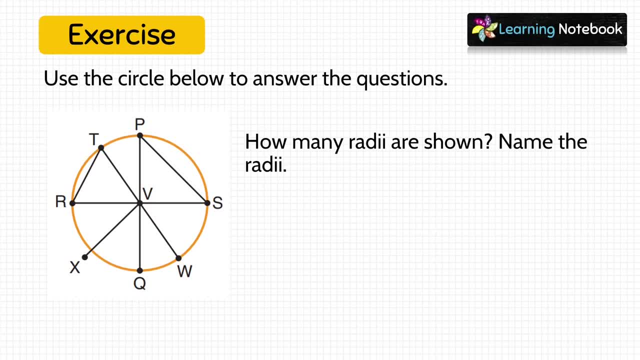 The plural of radius is radii. So let's look. So we have to look for radii here. So we have to look for line segments which have one endpoint at the center and other endpoint on the circle. So line segment VQ, VW, VS, VP, VT and VR. 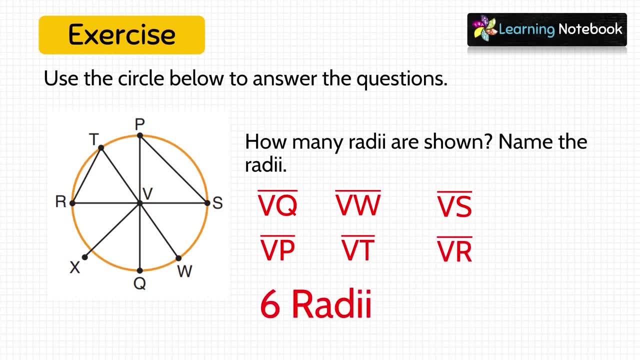 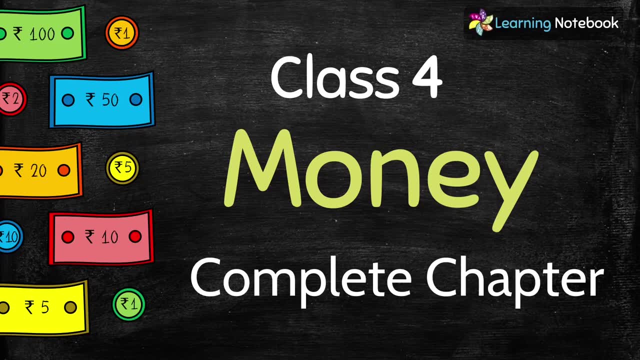 So these are segments. There are six radii shown in this circle: pie. ah, Students, we have a complete chapter of money for class 4.. I am sure all your doubts would be resolved after watching this video. The link to this video is here on the top and in the description box. 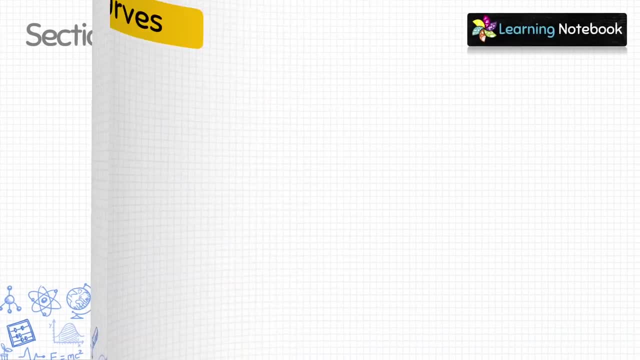 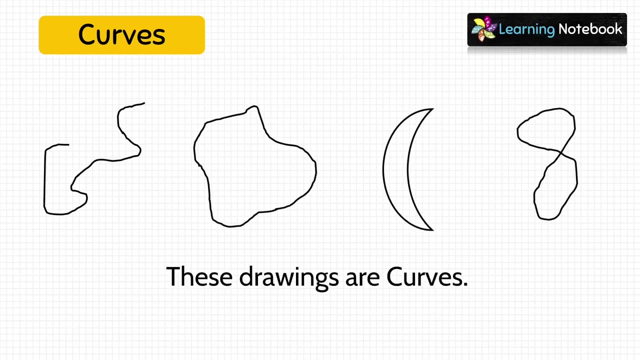 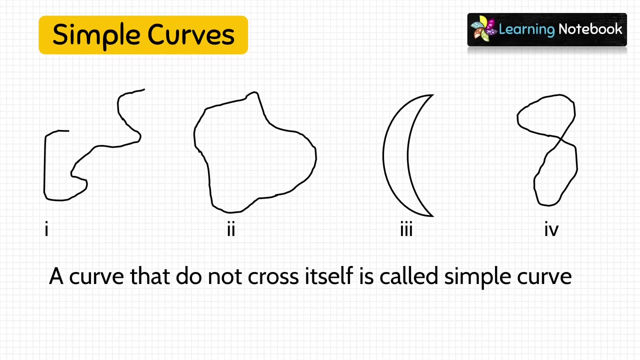 Now our next topic is curves and polygons. Students, you must have doodled on a piece of paper. Some of the results of these drawings are shown here on the screen. These drawings are called curves. So what are simple curves? A curve that do not cross itself is called a simple curve. So here, 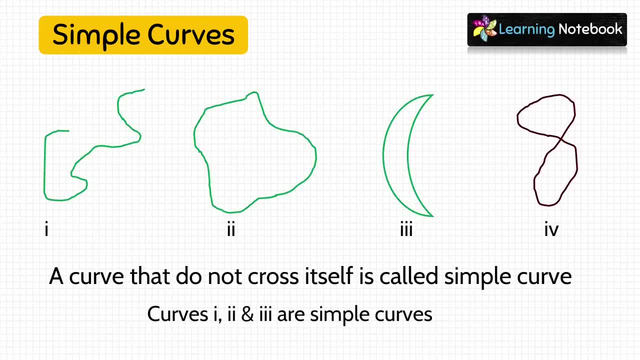 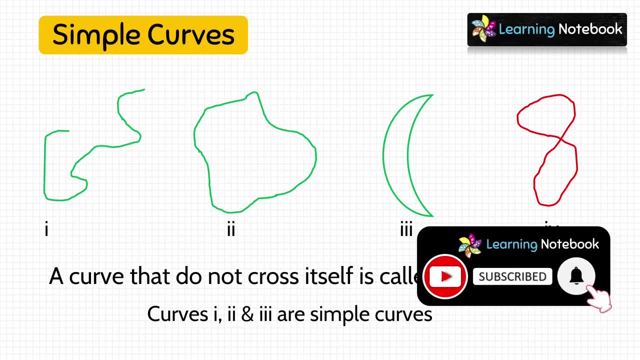 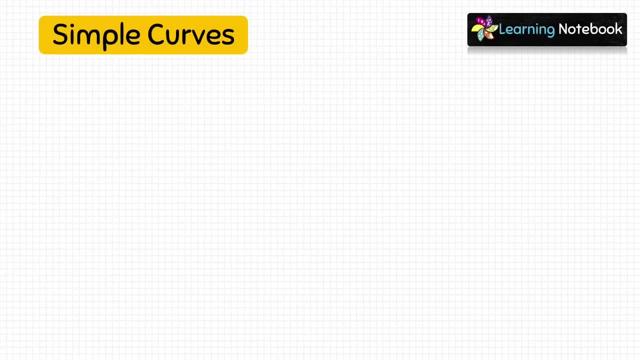 figure 1,, 2,, 3 are simple curves, But figure 4 is not a simple curve because it is crossing itself. Now, simple curves are of two types: open curves and closed curves. Open curves are the curves which do not end where they start. 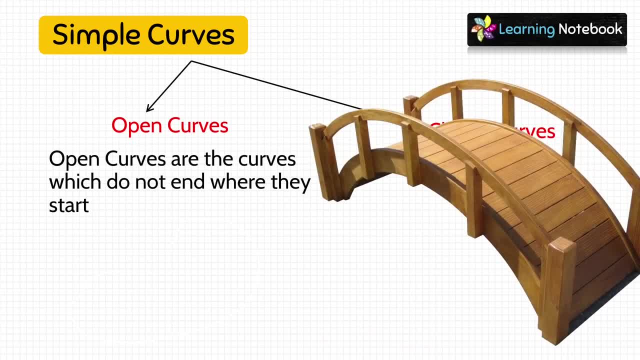 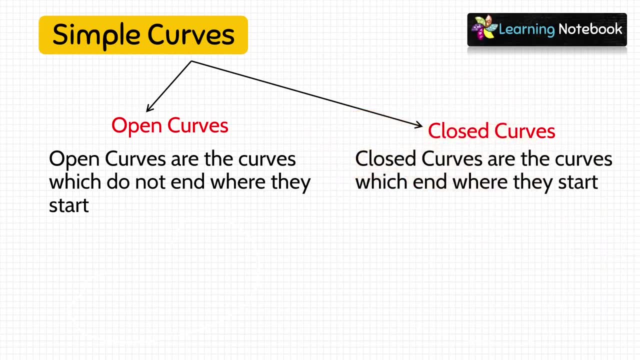 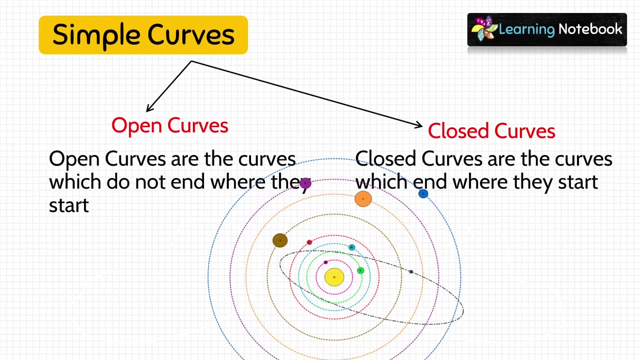 For example, curves of the bridge are perfect example of open curves. Closed curves are the curves which end where they start, For example, curves of orbiting planets. The orbits end where they start. So this is an example of closed curves. 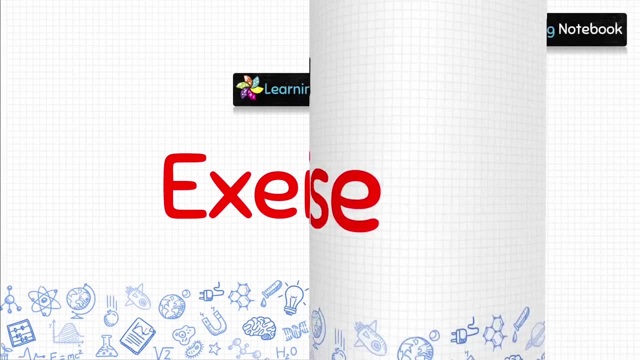 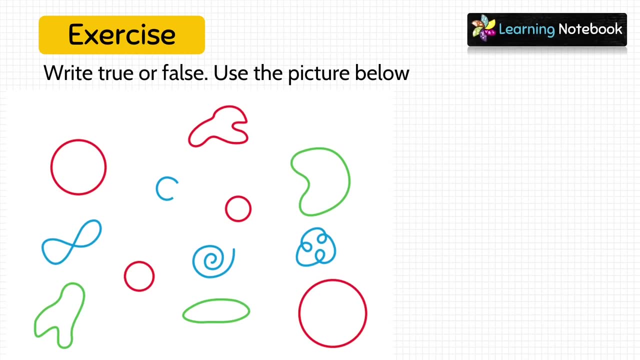 Now let's do an exercise based on curves. Write true or false. Use the picture below. The statement is: some of the simple closed curves are green. We know simple closed curves end where they start and they do not cross themselves. So yes, these are simple closed curves. 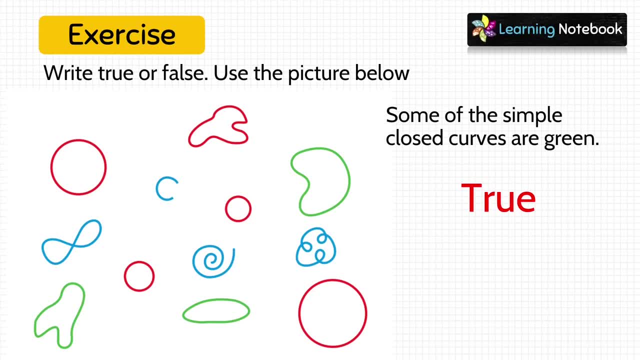 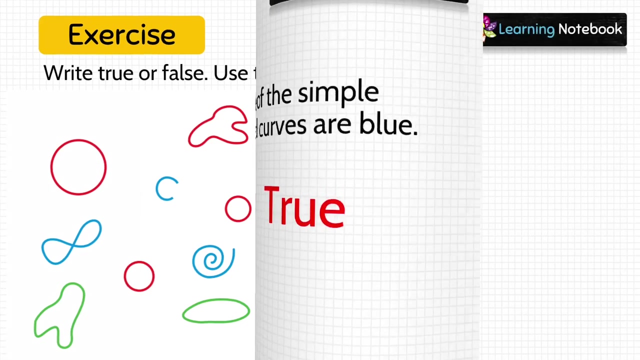 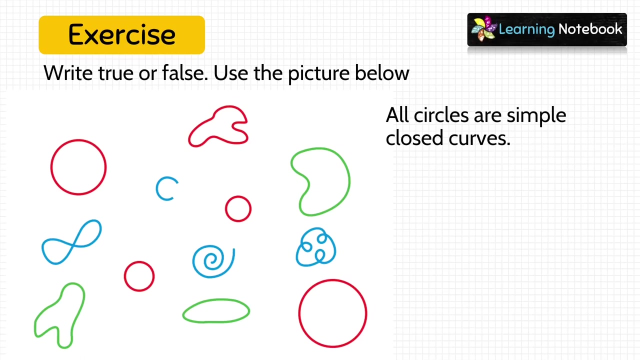 So the statement is true. Now, the second statement is: none of the simple closed curves are blue. So this statement is true, because some of them are crossing each other and some are not ending where they start. all circles are simple closed curves. 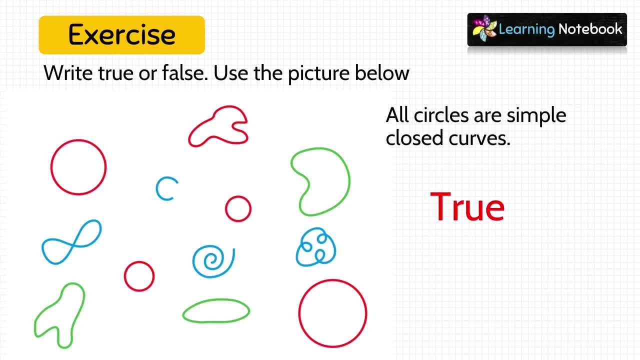 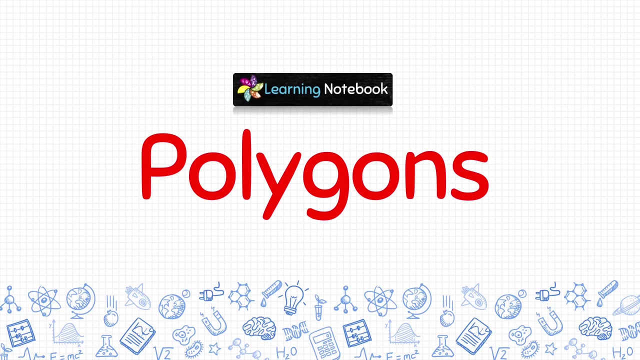 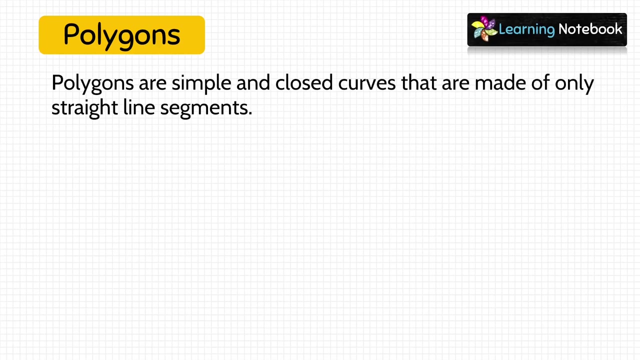 So this statement is also true. And the last statement is: none of the simple closed curves are red. This statement is false because all of the figures in red are simple closed curves. Now, students, our next topic is polygons. Polygons are simple and closed curves. 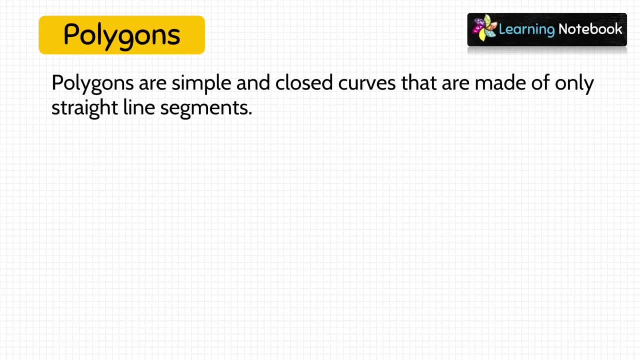 that are made of only straight line segments. Let's take few examples to understand polygons. This figure is a simple curve, closed curve, and is made of only line segments. So this is a polygon. Now let's take a look at the second example. 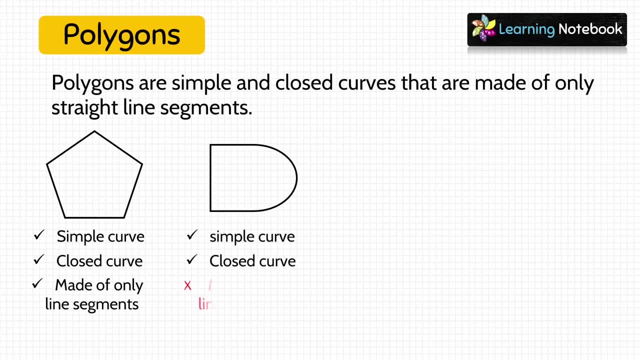 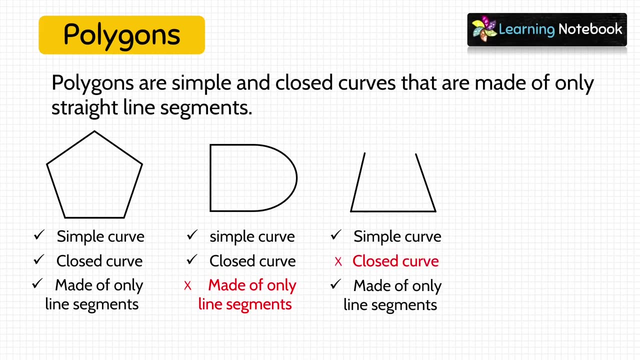 This figure is a simple curve, closed curve, but it is not made of only line segments, So this is not a polygon. Third figure: it is a simple curve made of only line segments, but it is not a closed curve, So it is not a polygon. 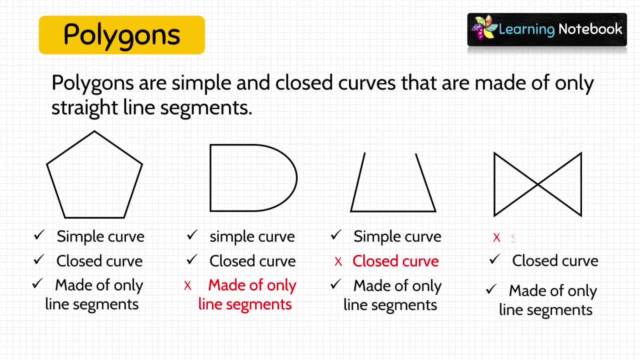 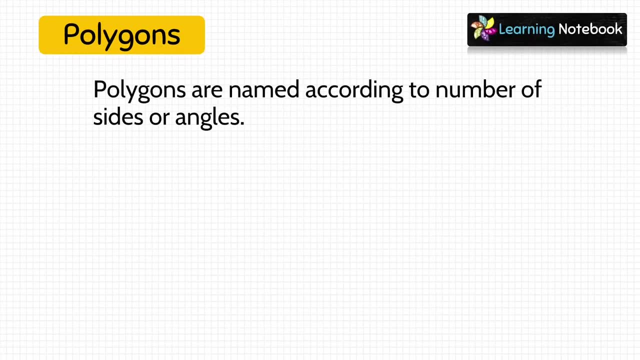 Now the last figure. it is a closed curve made of only line segments, but it is not a simple curve. So again, this is not a polygon. Polygons are named according to number of sides or angles. For example, polygon with three sides or three angles is called triangle. 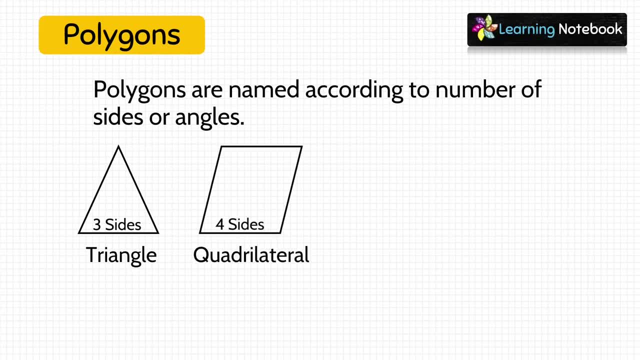 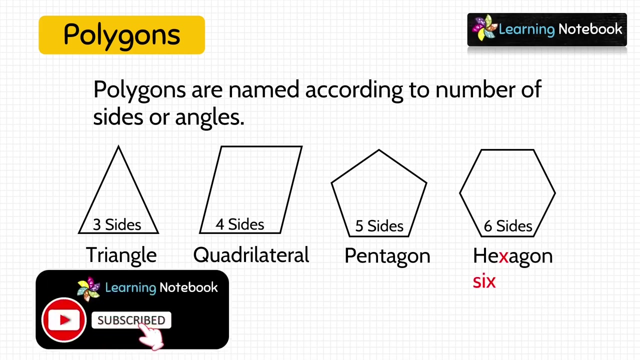 Polygon with four sides or four angles is called quadrilateral. Square and rectangle are examples of quadrilateral Polygon with five sides or five angles is called pentagon. Next polygon with six sides or six angles is called hexagon. You can easily remember hexagon from six. 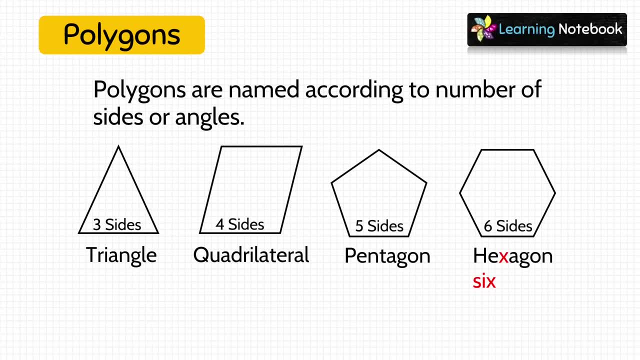 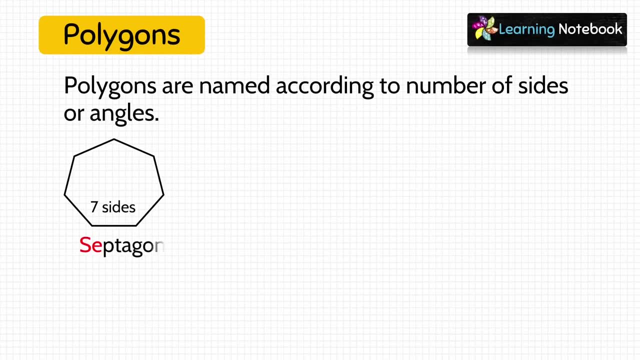 As both words hexagon and six are used for hexagons. As both words hexagon and six are used for hexagons. As both words hexagon and six are used for hexagons, 6 have letter X common. Now polygon with 7 sides or 7 angles is called. 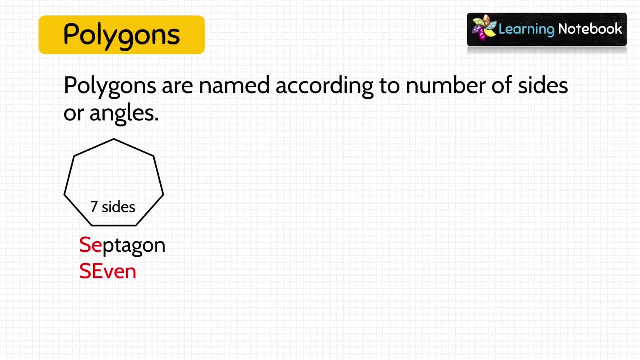 septagon. You can remember septagon from 7, as both words septagon and 7 have initial letters SE. Next, polygon with 8 sides or 8 angles is called octagon. You can remember octagon from word octopus, as we all know that an octopus has 8 arms. Next, a polygon with 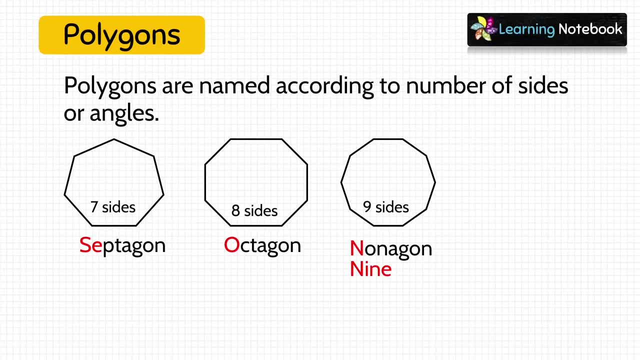 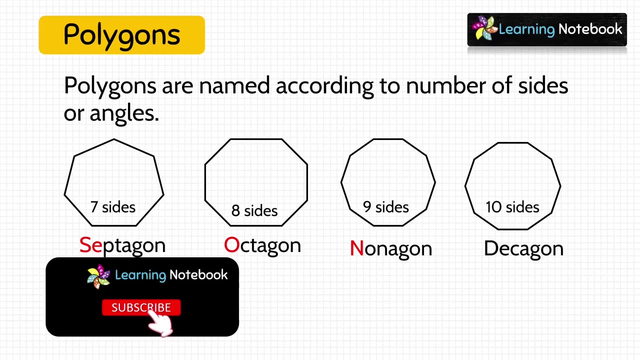 9 sides or 9 angles is called nonagon. You can easily remember it from 9, as both start from letter N. And lastly, a polygon with 10 sides or 10 angles is called decagon. So, students, in this video we learnt all. 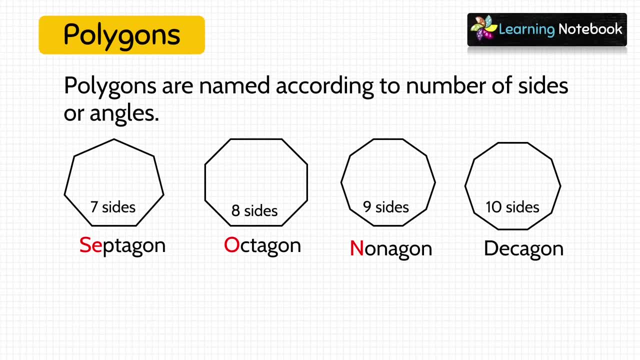 the concepts related to geometry, and we did lots of exercise on each of these concepts. If you enjoyed this video, then do share it further. Thanks for watching. See you in the next video. Bye-bye.